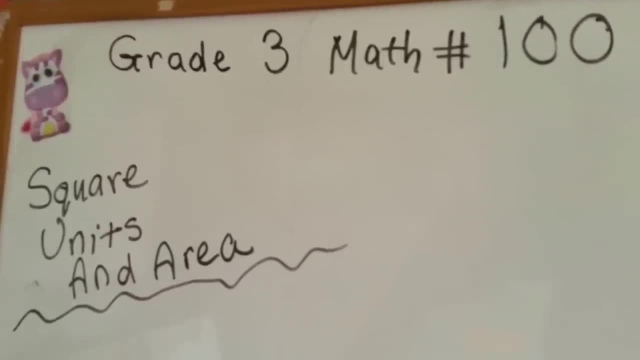 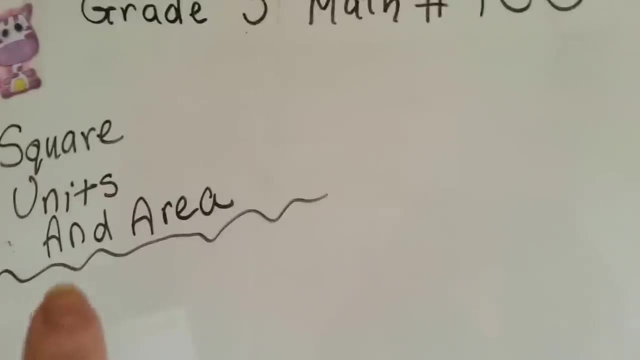 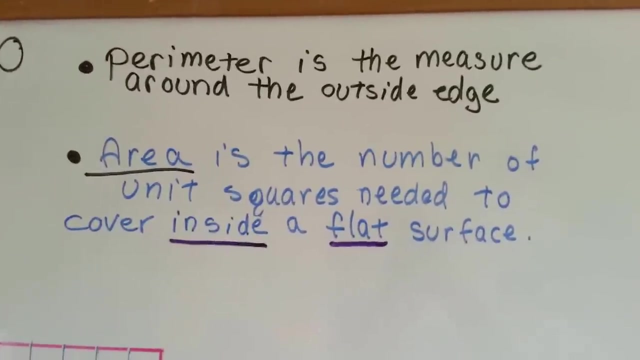 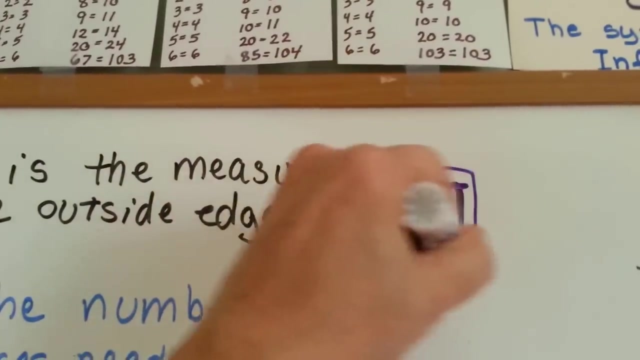 Grade 3 math, number 100.. Square units and area. We're also going to talk about units- square- Not to be confused with square units. Isn't that silly? Okay, if you remember from our other videos, perimeter is the measure around the outside edge of an object. So if you have a square or a shape, the perimeter is the measure going all the way around the outside of the object. Okay, 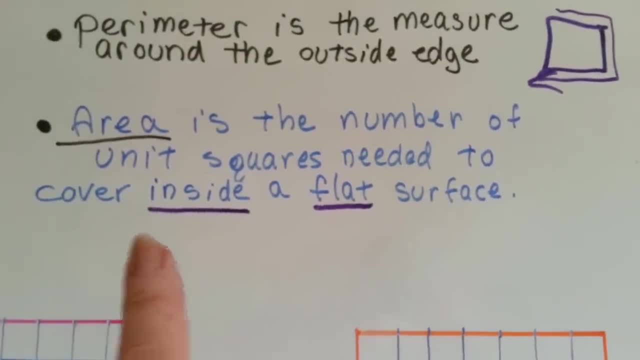 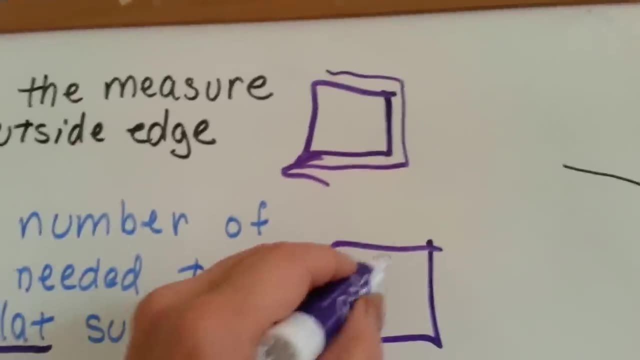 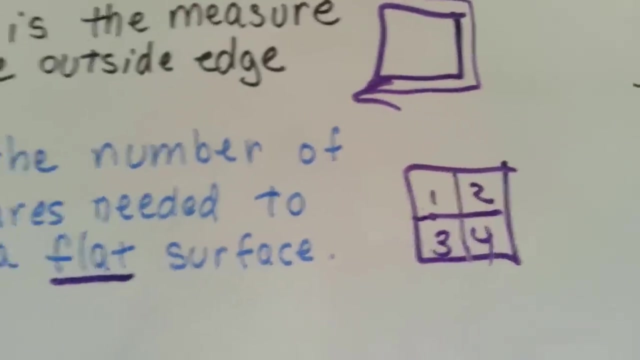 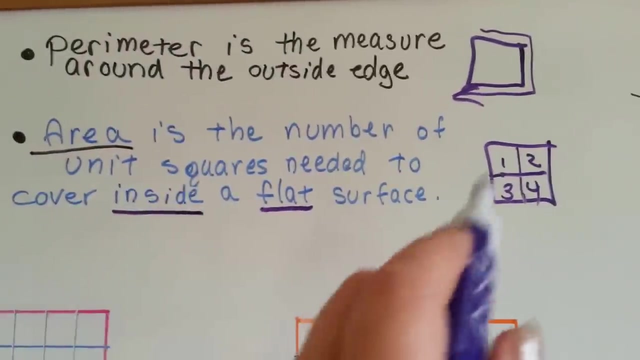 Area is the number of unit squares needed to cover the inside of the flat surface. So if you have this flat surface, how many unit squares do you need to fill it? This one would be four. That's its area. Whether it's four feet, four inches, four centimeters, we don't know. That's what a unit square is. It's an arbitrary amount. that is just one unit long. 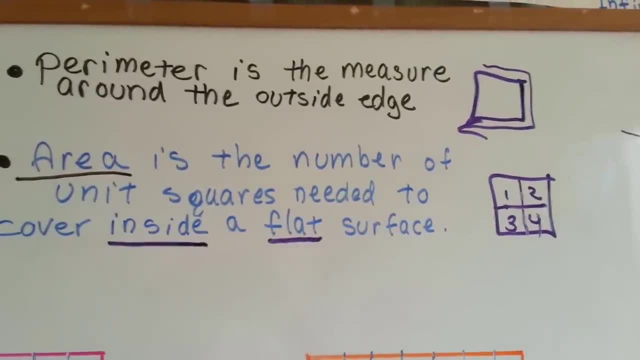 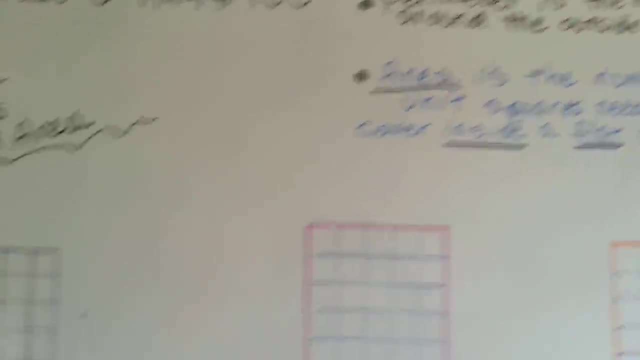 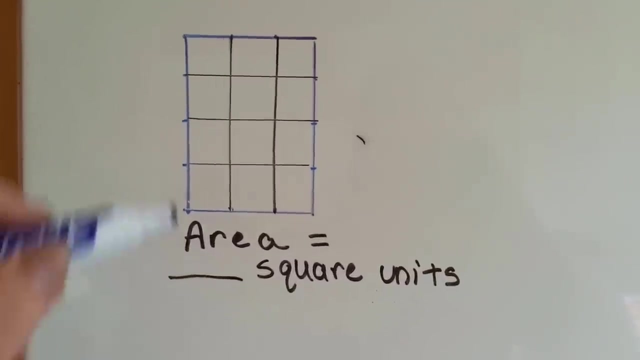 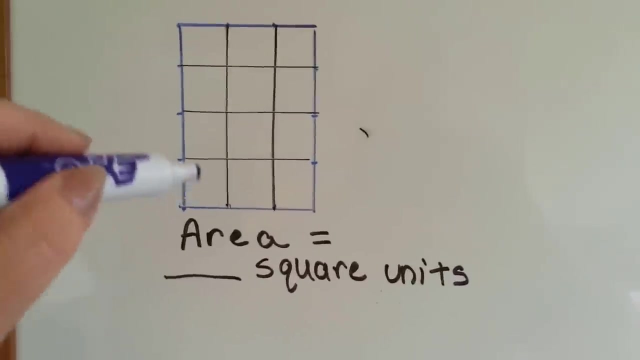 It could be paperclips, It could be crayons, It could be any length, but it would be one unit, one paperclip, one crayon. Okay, So that's the unit, All right. So if we were to look at a rectangle and we wanted to figure out what its area is, we would break it into its units and look to see how many squares are on the inside. Okay, 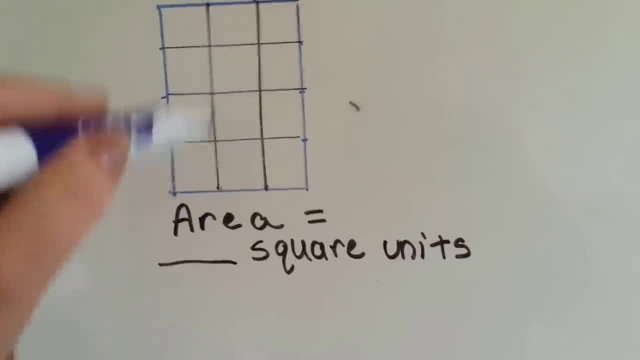 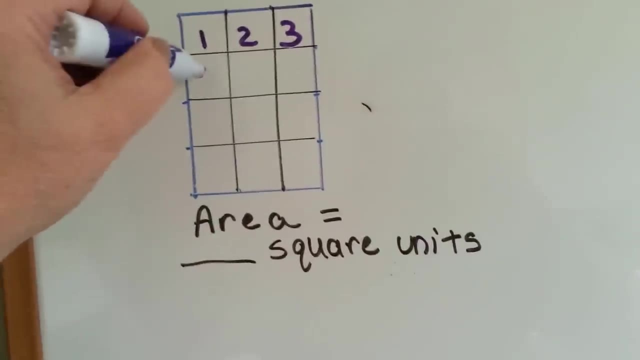 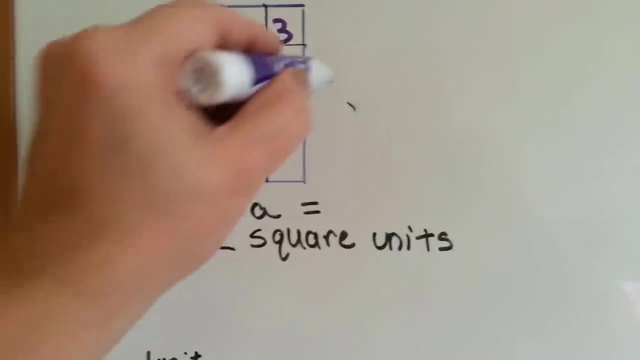 We're not counting the perimeter of the outside, we're counting how many of these squares are on the inside. there's three going across and four going down. So what we could do is we could say three times four. And what is three times four? 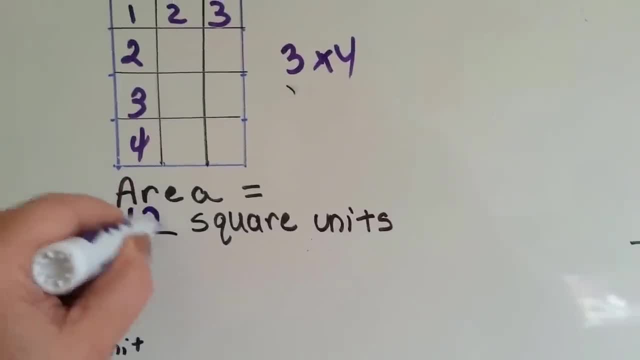 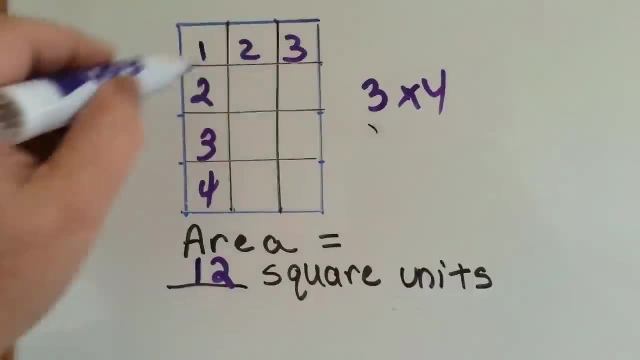 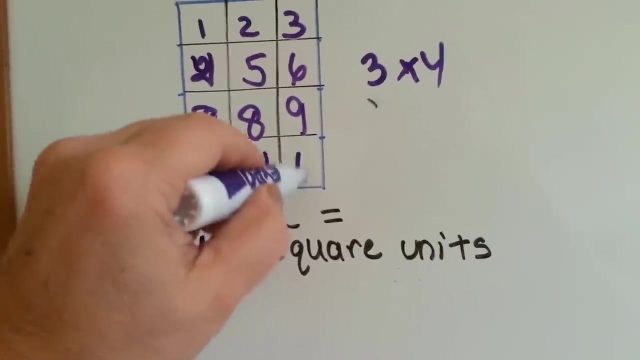 Do you remember? Three times four is twelve, So this rectangle has twelve square units. Now let's check it out. Does it really One, two, three, four, five, six, seven, eight, nine, ten, eleven, twelve? It does. 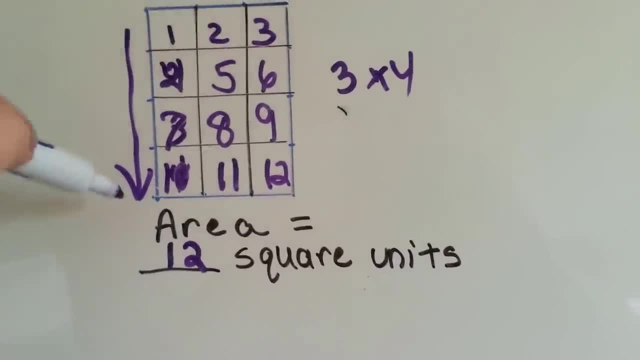 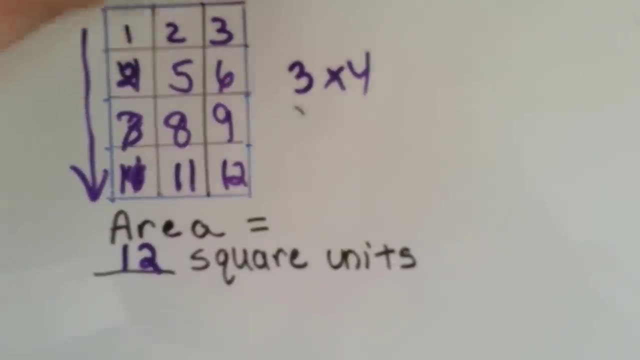 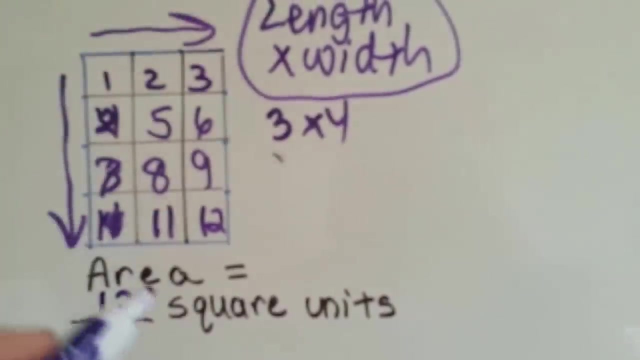 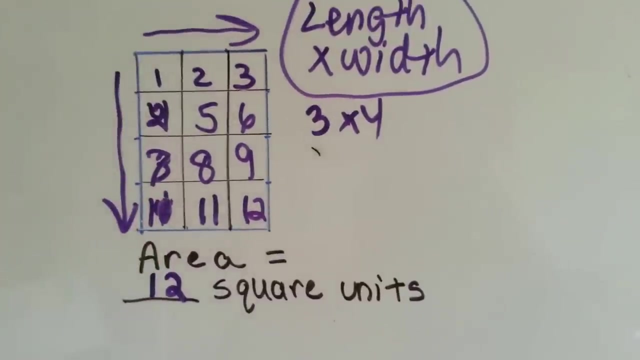 So if there's four coming down this way and three going that way, we could just do three times four. We could do the length times the width. And if we do the length times the width and it's a full shape that doesn't have any indentations like a U-shape or anything, 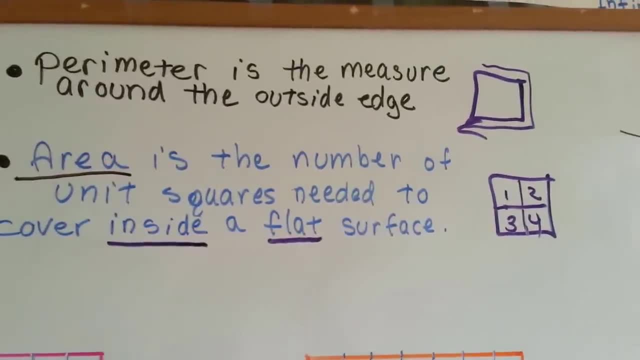 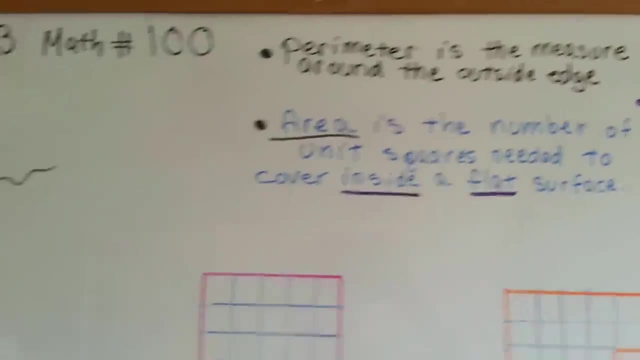 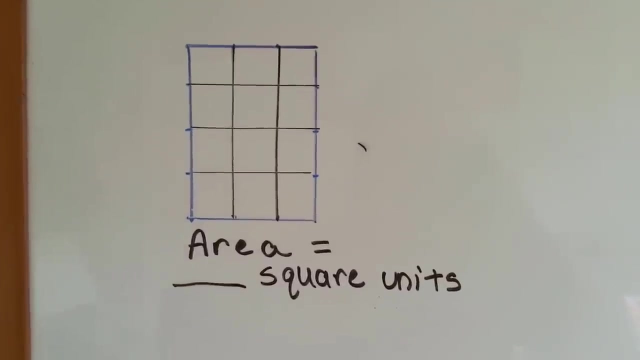 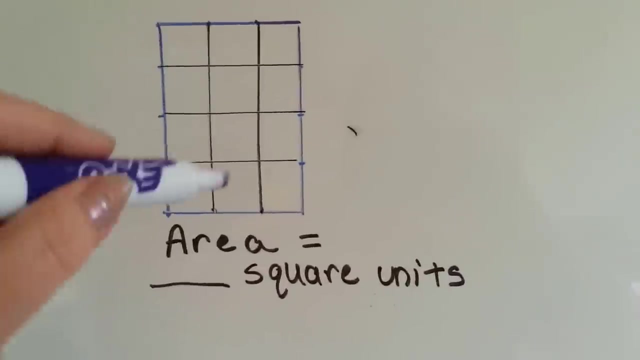 It could be paperclips, It could be crayons, It could be any length, But it would be one unit, one paperclip, one crayon. Okay, So that's the unit, Alright. So if we were to look at a rectangle and we wanted to figure out what its area is, we would break it into its units and look to see how many squares are on the inside. Okay, 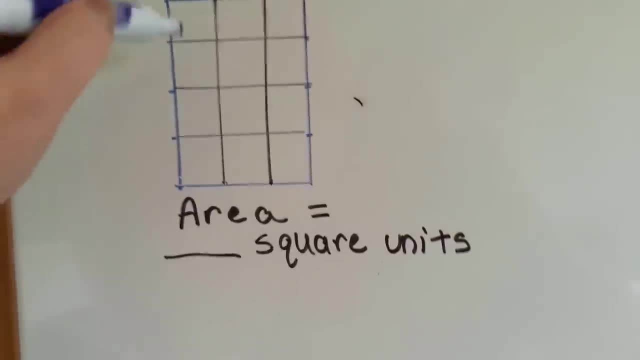 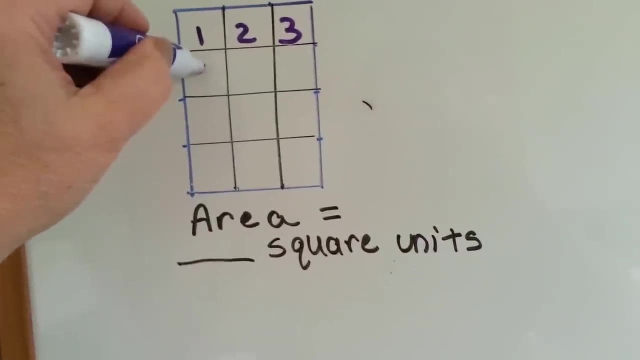 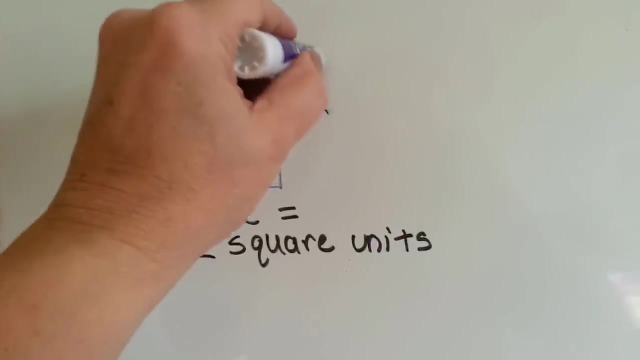 We're not counting the perimeter of the outside. We're counting how many of these squares are on the inside squares are on the inside. there's 3 going across and 4 going down. So what we could do is we could say 3 times 4.. 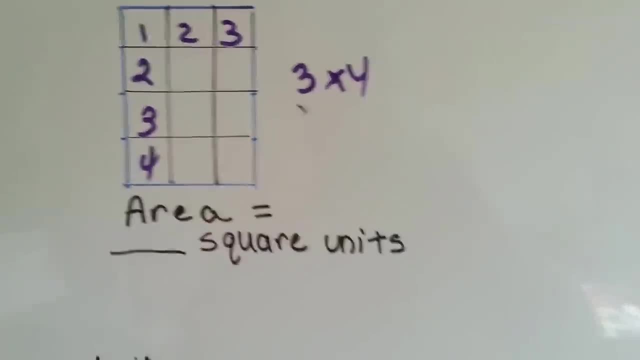 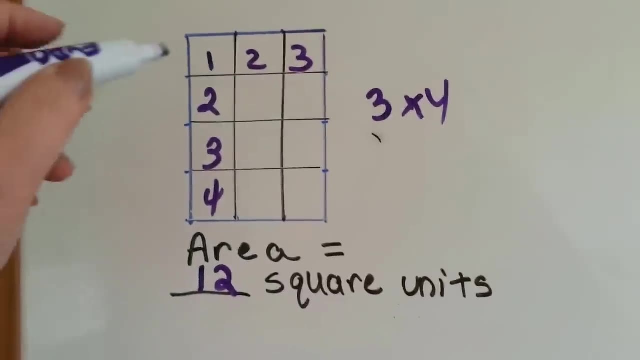 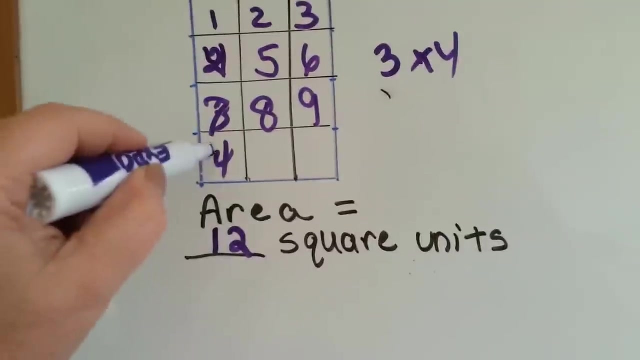 And what is 3 times 4?? Do you remember? 3 times 4 is 12.. So this rectangle has 12 square units. Now let's check it out. Does it really 1, 2, 3, 4, 5, 6, 7,, 8, 9,, 10,, 11,, 12.? 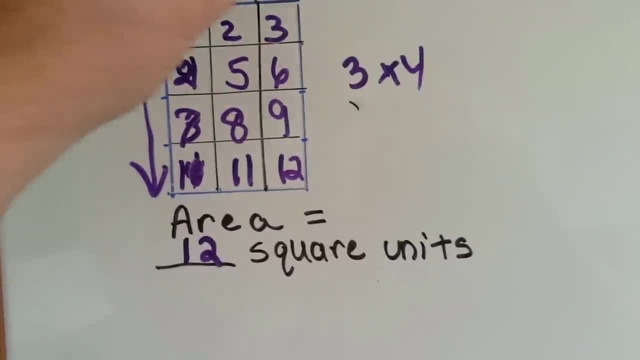 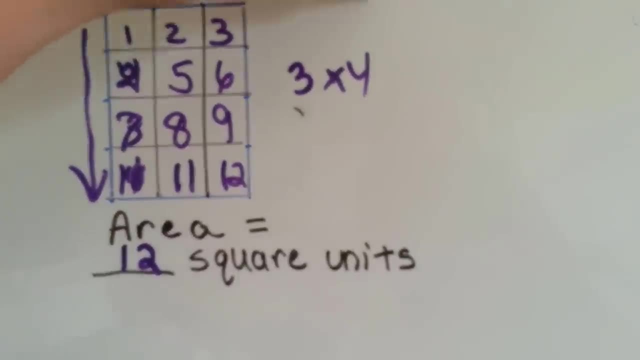 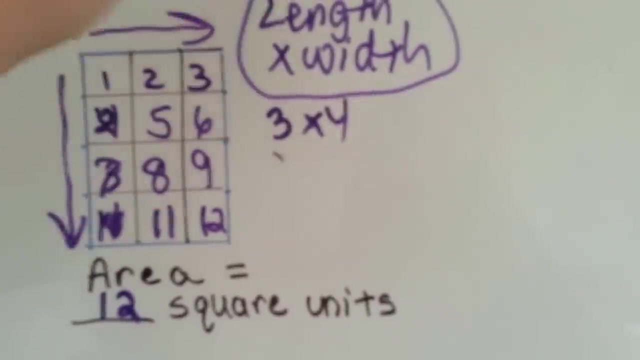 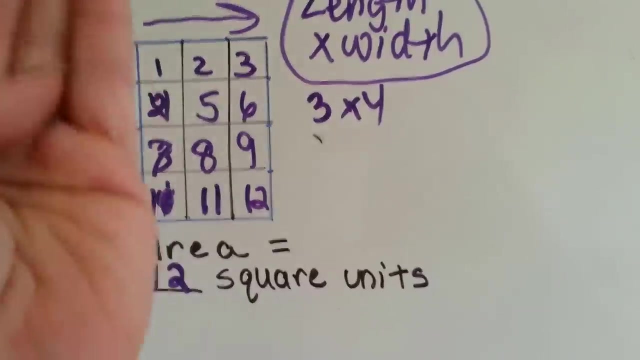 It does. So if there's 4 coming down this way and 3 going that way, we could just do 3 times 4.. We could do the length times the width, And if we do the length times the width And it's a full shape that doesn't have any indentations, like a U shape or anything, 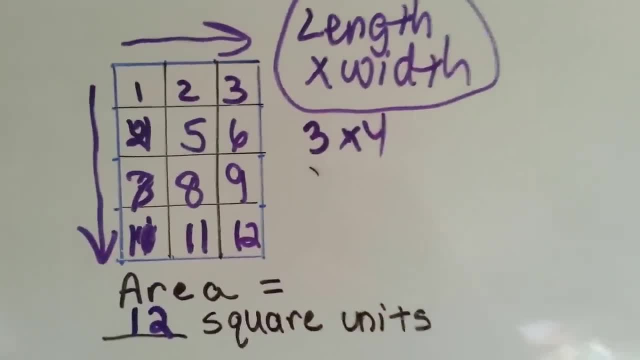 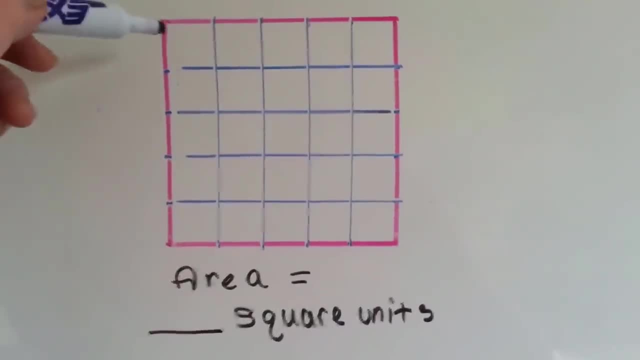 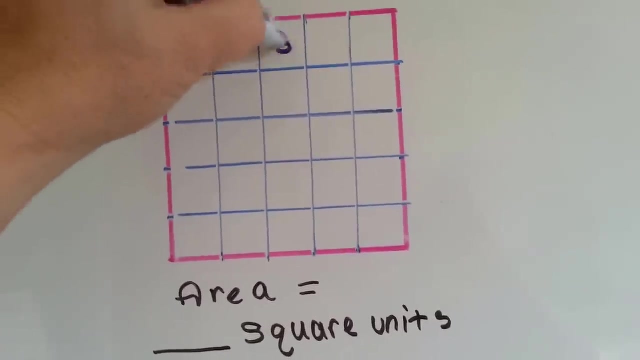 If we wanted a full shape like this, we could do length times width. So now let's look at this one. Let's find the area of this one. How many universal units, squares, are going across this way? 1,, 2,, 3,, 4, a, 5.. 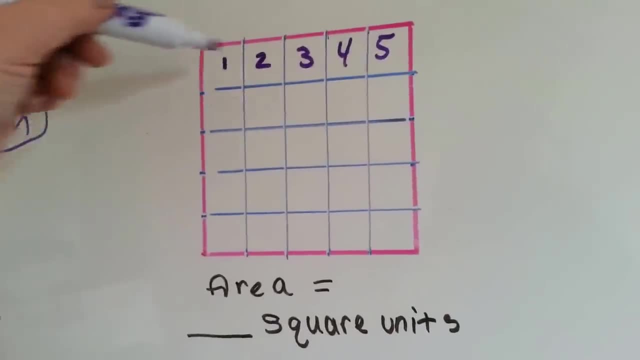 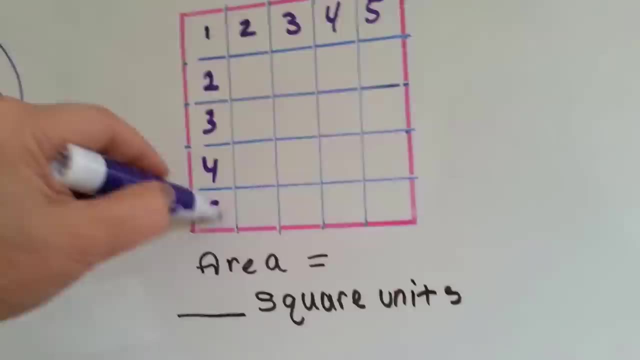 Ok, 5.. Five, One. So it's a full line. Let's see where this goes. OK, Legs, How many are coming down the side? 1,, 2,, 3,, 4, 5.. So the length times the width would be 5 times 5.. 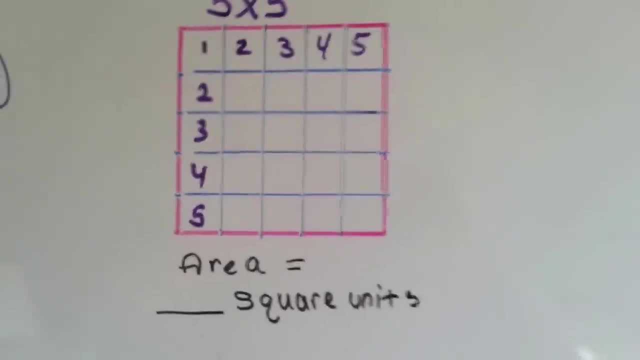 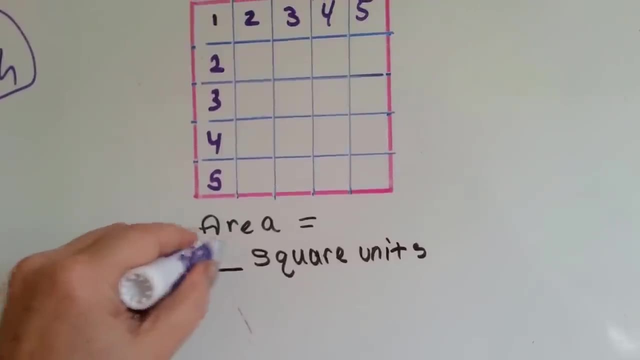 And what is 5 times 5?? Do you know? Have you memorized your times table yet, or at least your 5's, 5, 10,, 15,, 20,, 25.. So there's 25 square units here. Let's double check to see if we got it right. 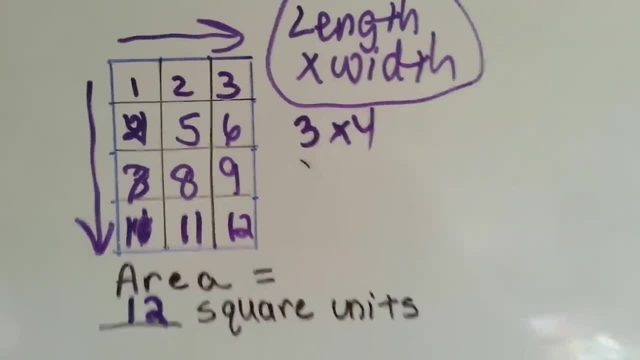 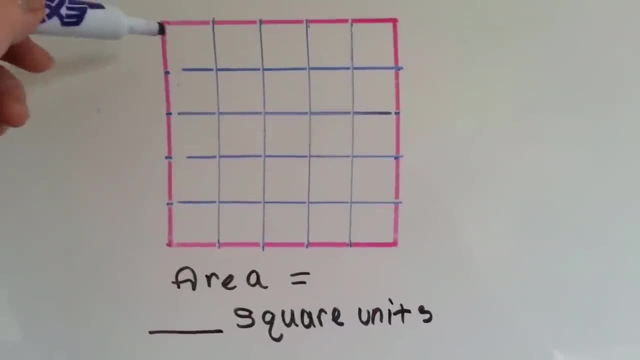 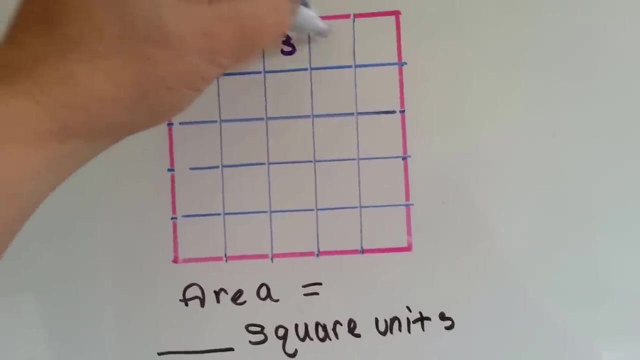 if it's a full shape like this, we can do length times, width. So let's look at this one, Let's find the area of this one. How many boxes, how many unit squares are going across this way? One, two, three, four, five? 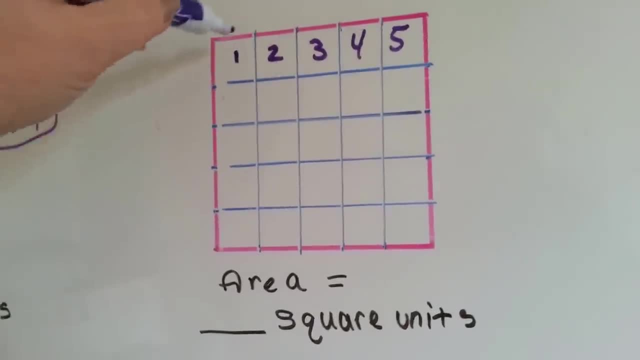 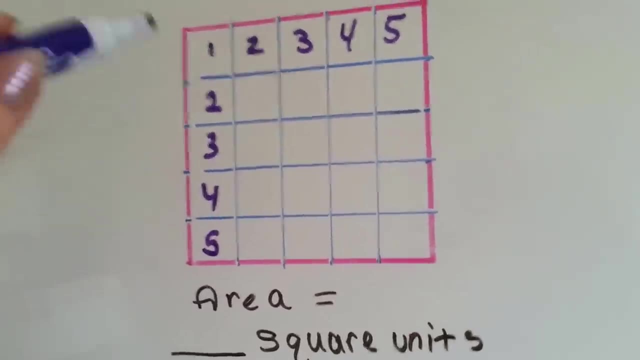 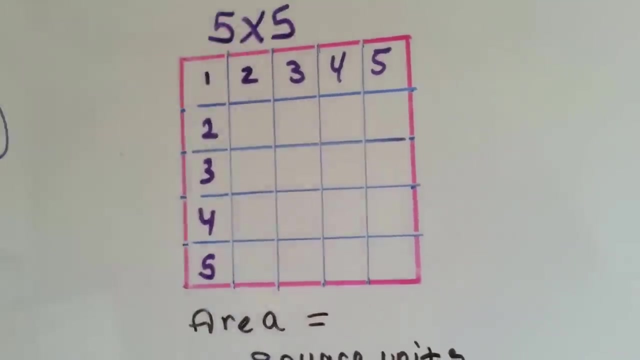 So we have five unit squares going across this way. How many are coming down the side? One, two, three, four, five. So the length times the width would be five times five. And what is five times five, Do you know? 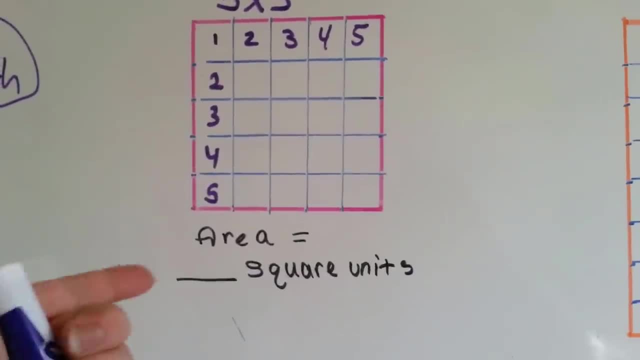 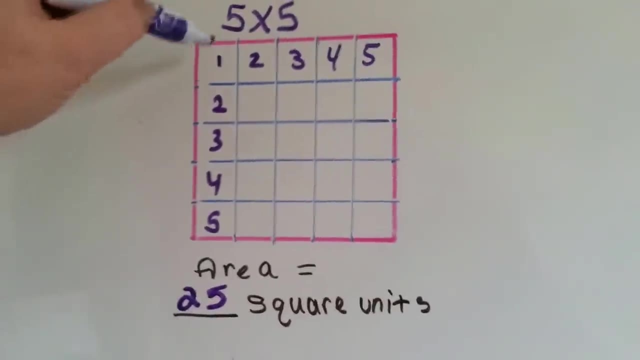 Have you memorized your times table yet, or at least your fives? Five, ten, fifteen, twenty, twenty-five. So there's twenty-five square units here. Let's double check to see if we got it right. That's five. 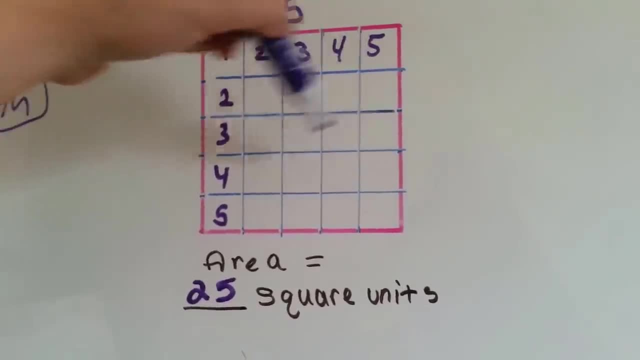 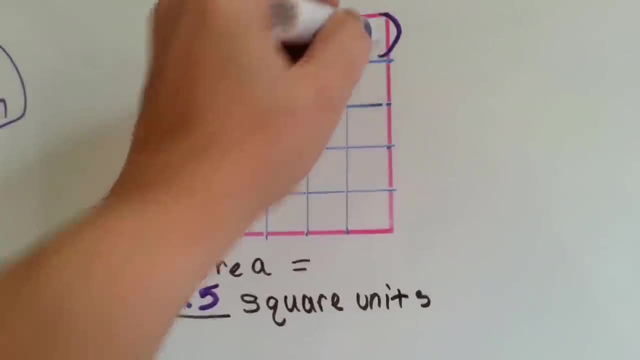 six, seven, eight, nine, ten, eleven, twelve, thirteen, fourteen, fifteen, sixteen, seventeen, eighteen, nineteen, twenty, twenty-one, twenty-two, twenty-three, twenty-four, twenty-five. Here's a group of five. 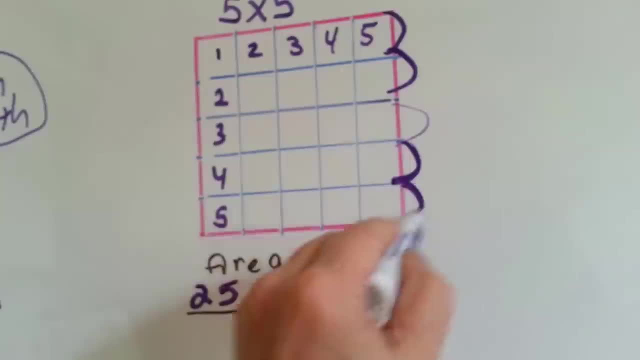 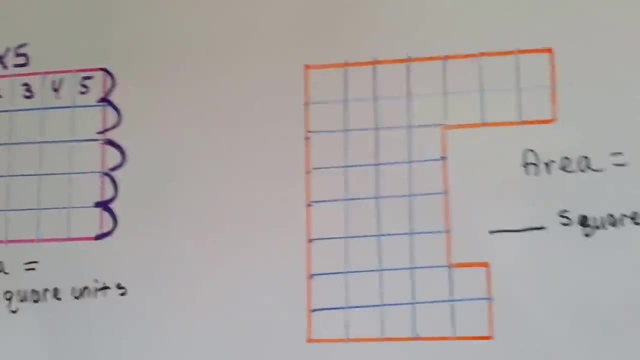 here's a group of five, here's another one, and another one, and another one. So we have five groups of five, that's twenty-five square units. So now let's look at the units and the area on this odd shape. Now we can't do length times width on this one. 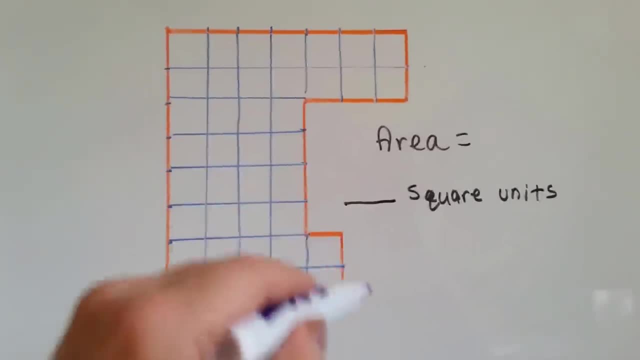 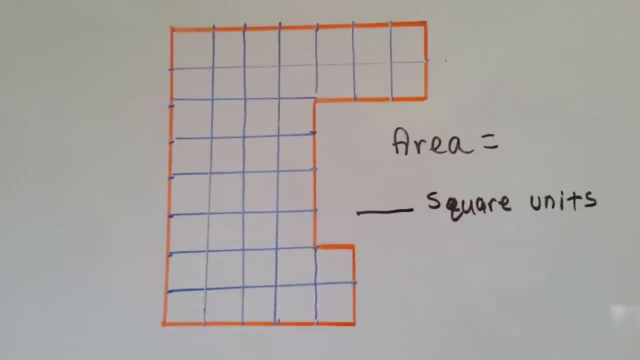 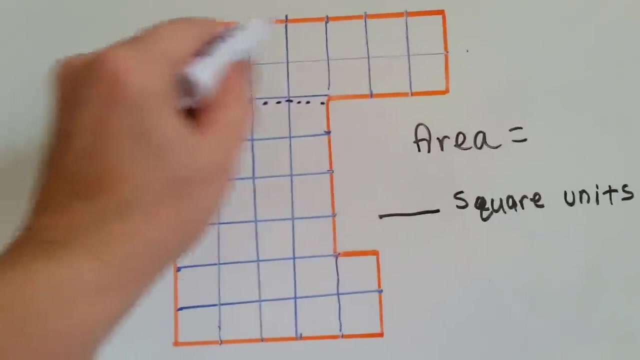 the way we did it over here, Because, look, there's part of the shape missing, So it wouldn't be the same as this one that's all full. So what we could do is we could break it into smaller pieces and do the length and the width on this one. 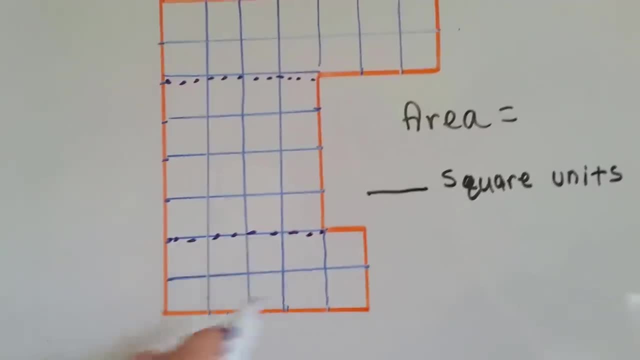 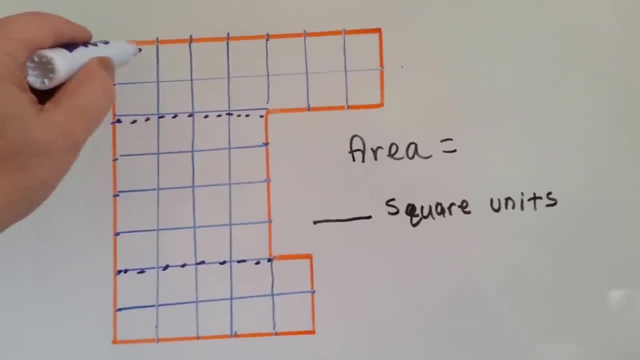 do the length and the width on the square in the center and then do the length and the width on this one See And then add them all up together. Okay, So this one is one, two, three, four, five, six, seven across. 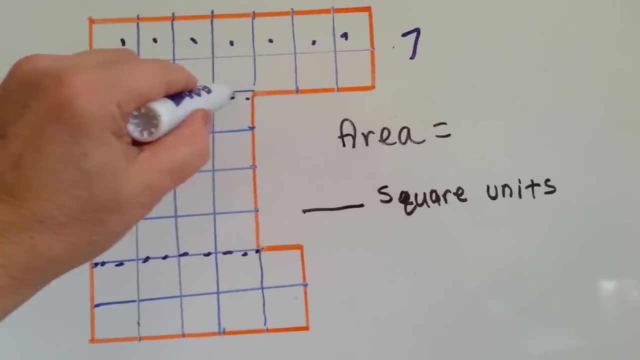 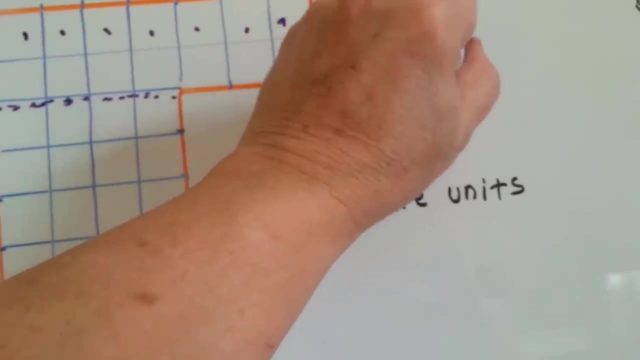 And how high is it? Now we're going to stop right here. remember, We're just going to do this top part. There's two, So we can say seven times two, which is fourteen, right? So let's put our fourteen right here. 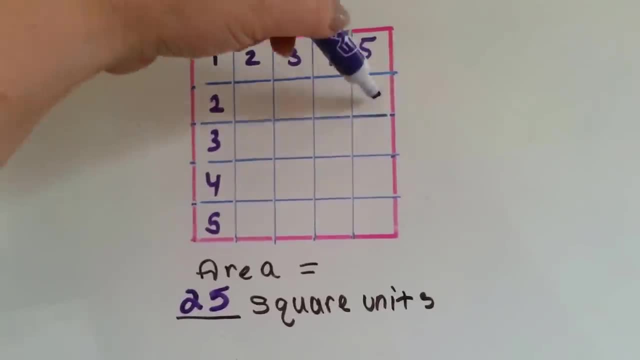 Okay, that's 5,, 6,, 7,, 8,, 9,, 10,, 11,, 12,, 13,, 14,, 15,, 16,, 17,, 18,, 19,, 20,, 21,, 22,, 23,, 24,, 25.. 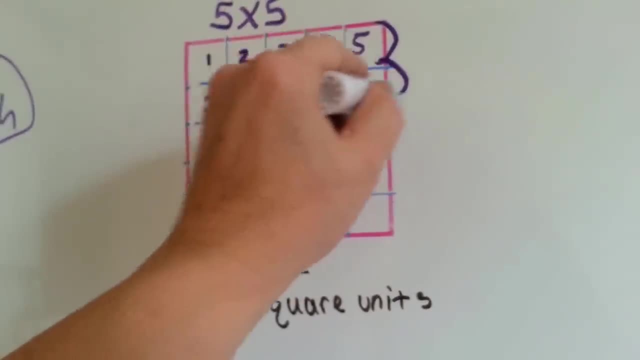 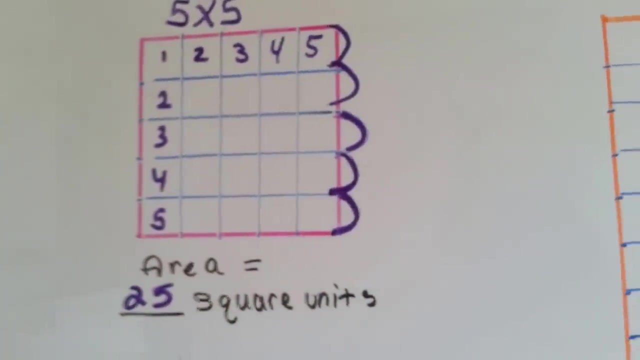 See, Here's a group of 5, here's a group of 5, here's another one, and another one, and another one. So we have 5 groups of 5, that's 25 square units. okay, So now let's look at the units and the area on this odd shape. 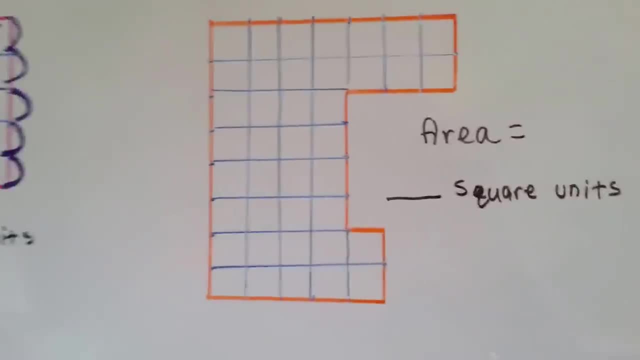 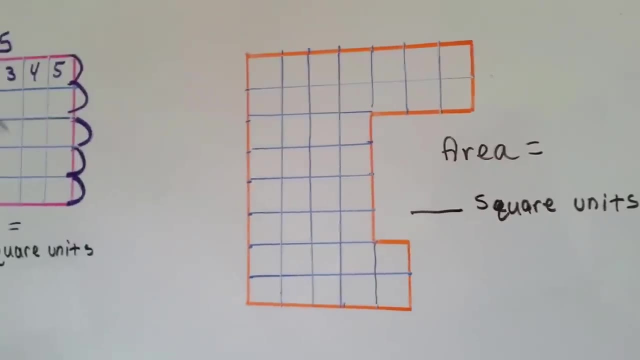 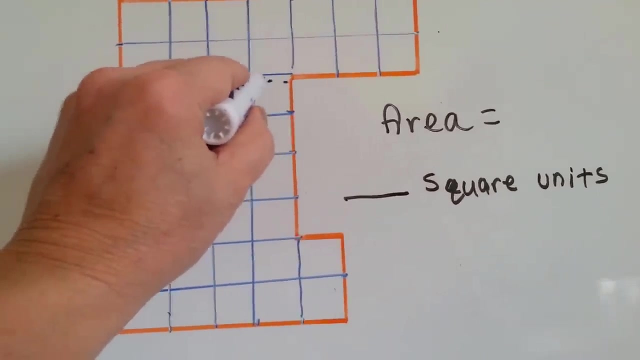 Now we can't do length times width on this This one the way we did it over here, because, look, there's part of the shape missing. okay, So it wouldn't be the same as this one. that's all full. So what we could do is we could break it into smaller pieces. 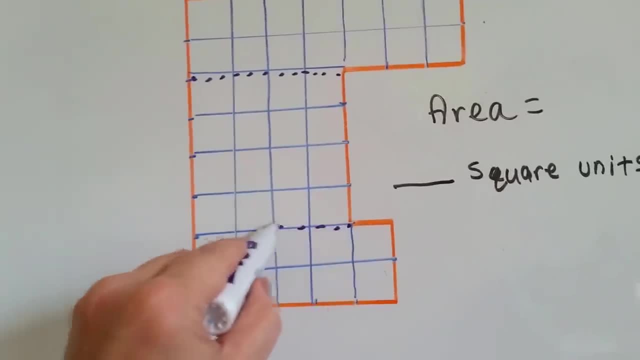 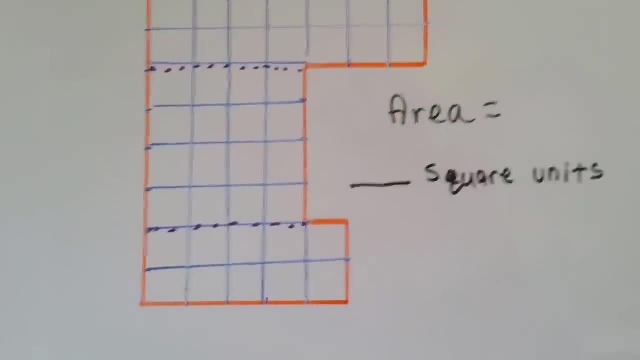 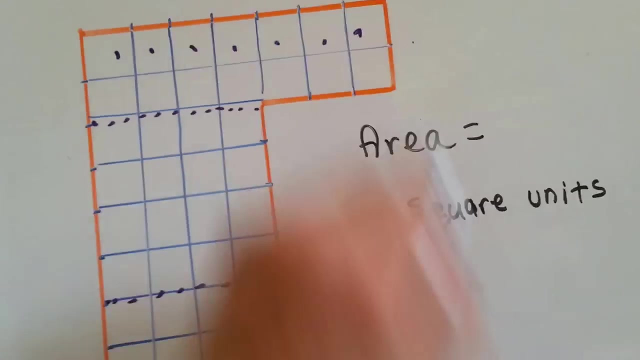 and do the length and the width on this one, Do the length and the width on the square in the center and then do the length and the width on this one, See, And then add them all up together. Okay, So this one is 1,, 2,, 3,, 4,, 5,, 6,, 7, across, and how high is it? 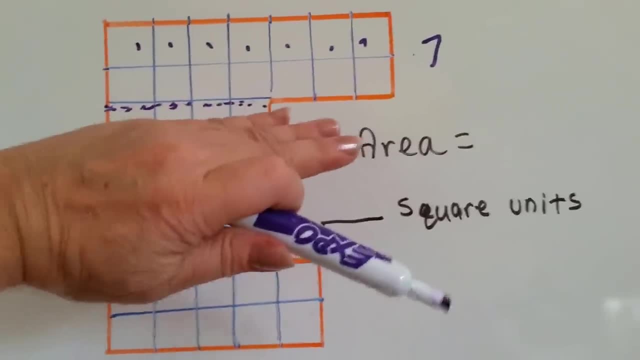 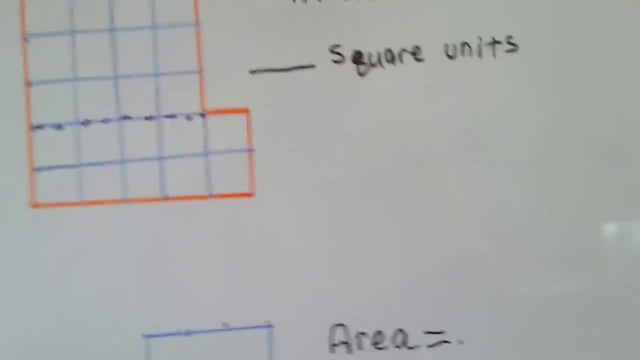 Now we're going to stop right here. remember, We're just going to do this top part. There's 2, so we can say 7 times 2, which is 14, right? So let's put our 14 right here. 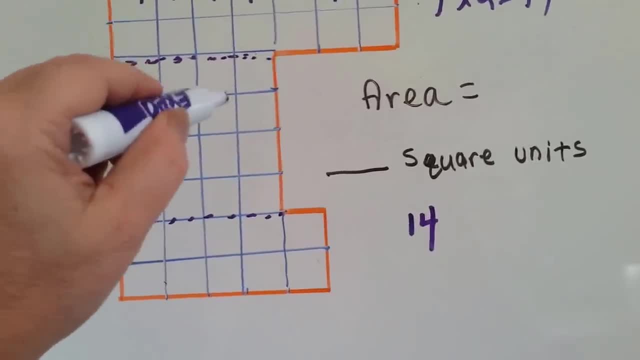 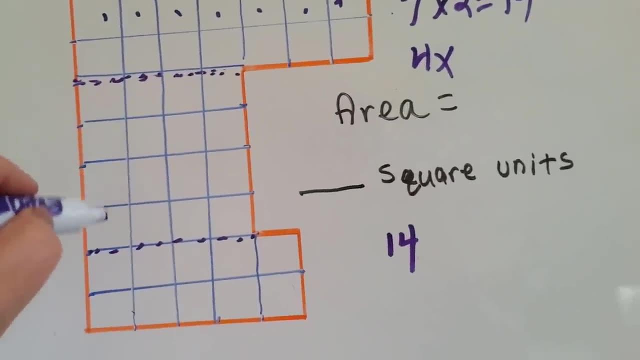 How big is this one? 1,, 2,, 3,, 4, across, okay, And how many is it coming down? 1, 2,, 3,, 4 coming down 4 times 4 is 16.. 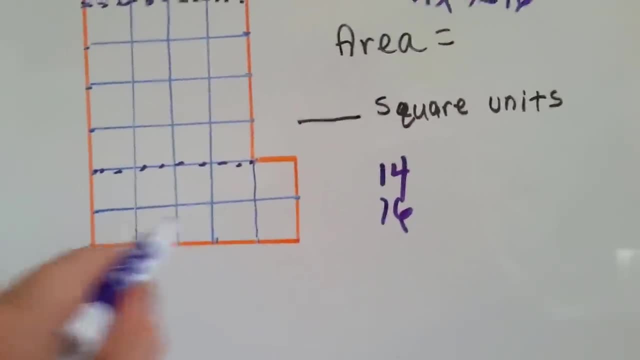 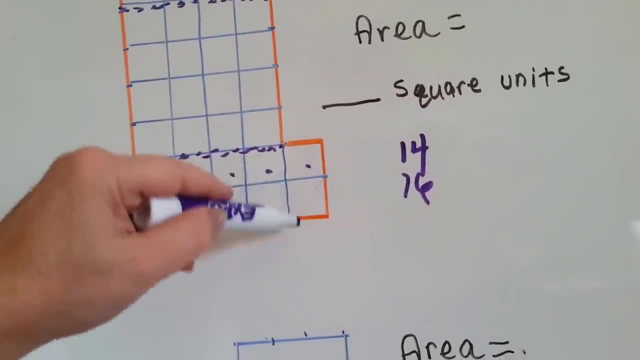 So now we're going to add 16 more to the big shape. And how many is the bottom part? Because, remember, we stopped here. We've got 1,, 2,, 3,, 4,, 5, and it's got the height of 2.. 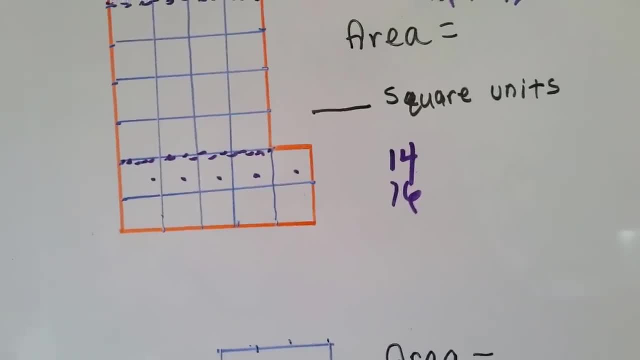 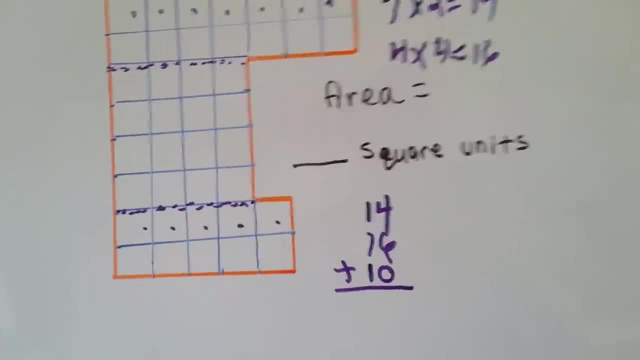 And what is 5 times 2?? 5 times 2 is 10.. So let's add that to our total. Now, let's add this up And it's going to tell us how much is in the whole thing. okay. 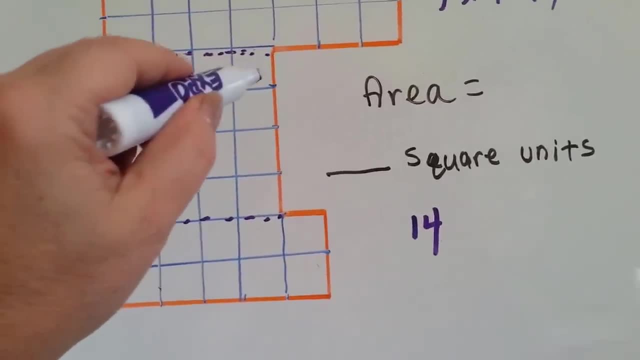 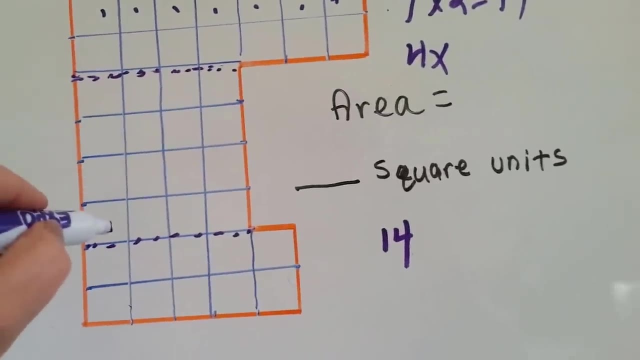 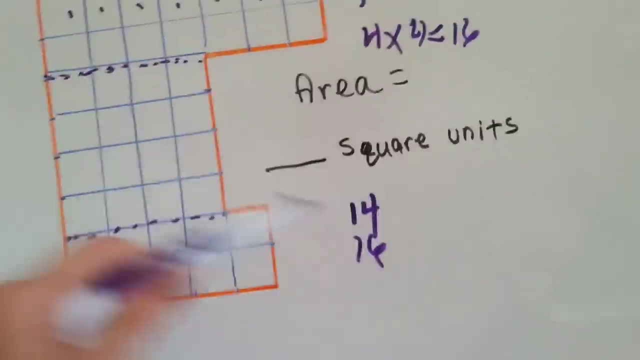 How big is this? one, One, two, three, four across, Okay, And how many is it coming down? One, two, three, four. coming down Four times four is sixteen. So now we're going to add sixteen more to the big shape. 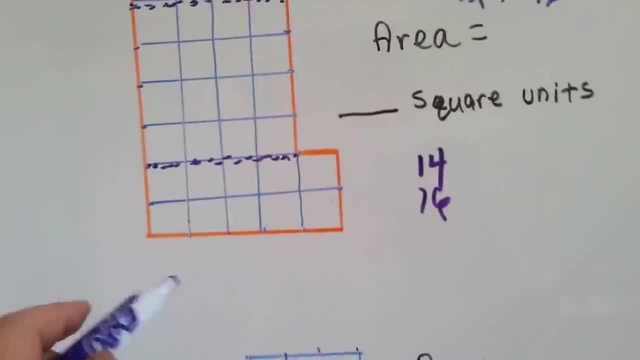 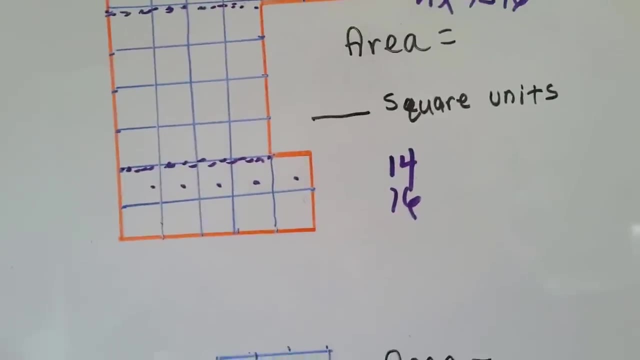 And how many is the bottom part, Because, remember, we stopped here. We've got one, two, three, four, five and it's got the height of two And what is five times two? Five times two is ten, So let's add that to our total. 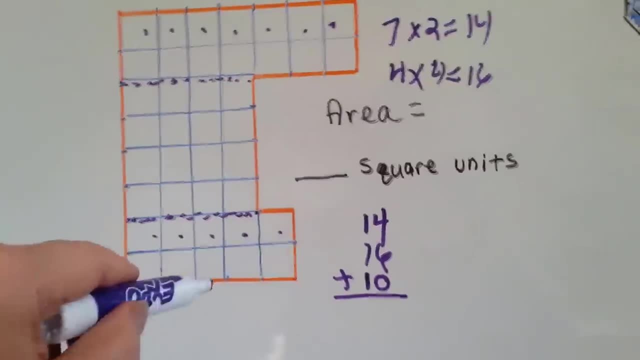 Now, let's add this up and that'll tell us how much it is. Now, let's add this up and that'll tell us how much it is. Now, let's add this up and that'll tell us how much it is. tell us how much is in the whole thing. Okay, 4 and 6 is 10.. We're going to carry the 1. 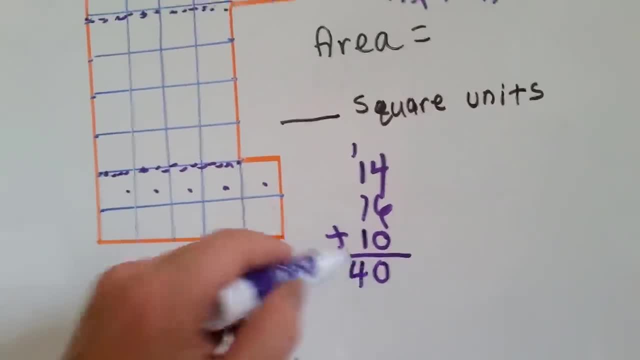 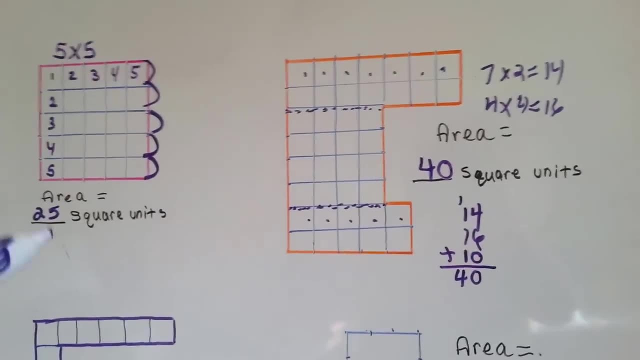 and put the 0 down: 1,, 2,, 3, 4.. There's 40 square units here. See Now, remember we weren't able to just do length times width like this one, because it was all full. This one's got. 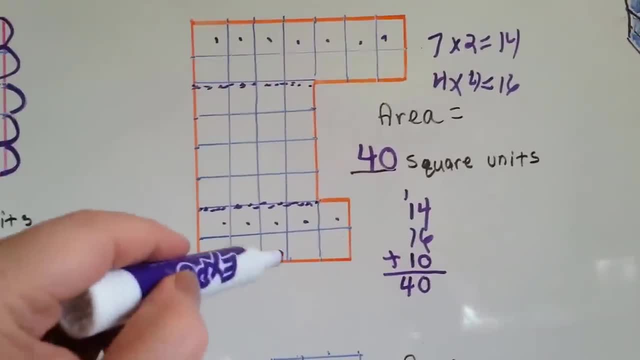 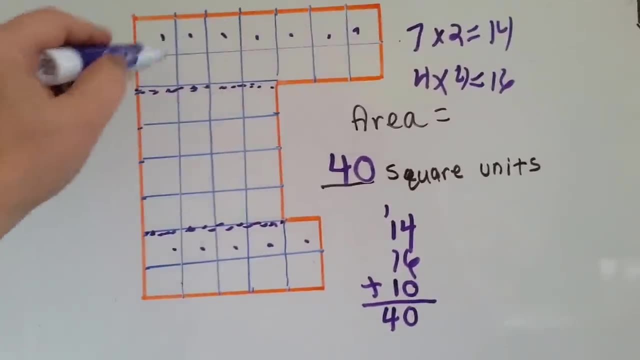 a missing space here. So what we did was we broke it into sections and did it that way. Now we didn't even have to do times table. We could have just added up, you know, 7,, 8,, 9,, 10,, 11,, 12,, 13,, 14.. We could have done it this way and counted each one of these. 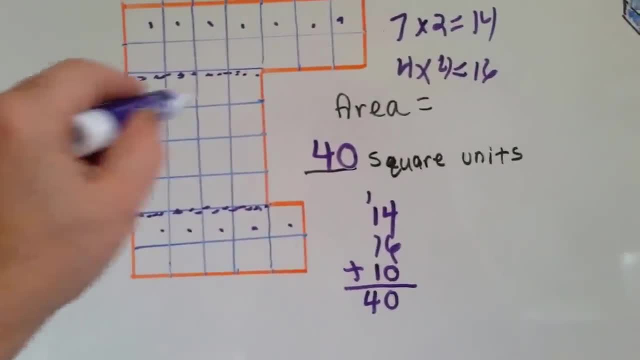 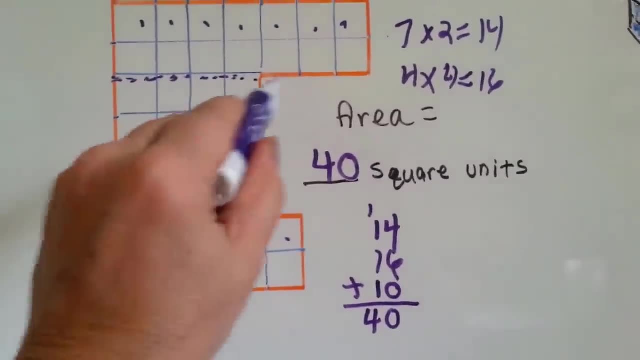 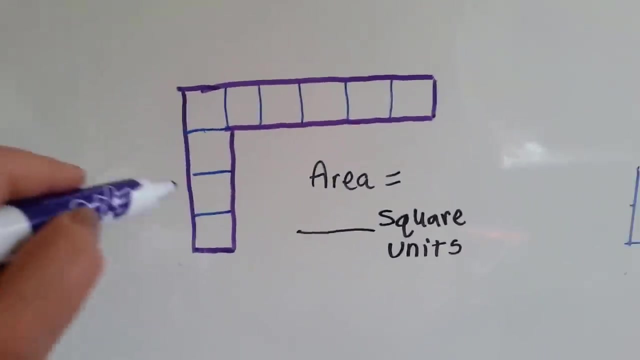 separately. It's just a little quicker to go like this and like this with the length and the width and multiply it and then get the amount. Just make sure that you break it off wherever it looks like it's changing. Okay, Now let's look at this over here. What? 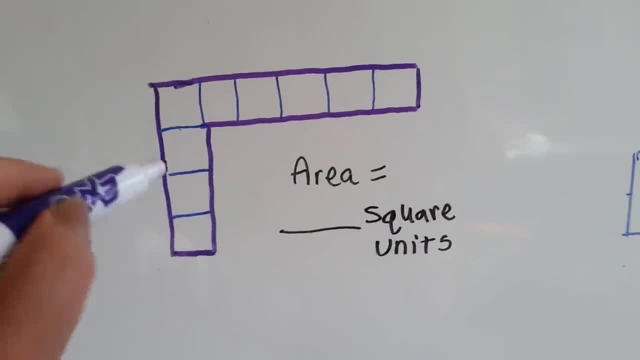 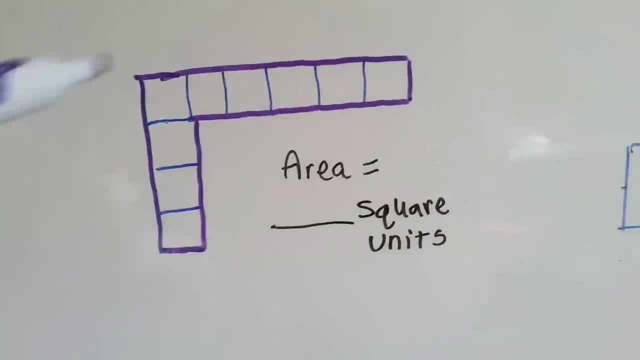 is the area of this? What are the unit squares? This one's got 1,, 2,, 3,, 4,, 5,, 6,, 7,, 8,, 9.. 9 square units And this one we were just able to count because it's in. 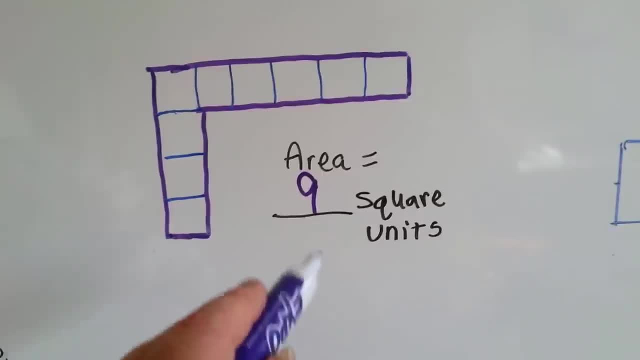 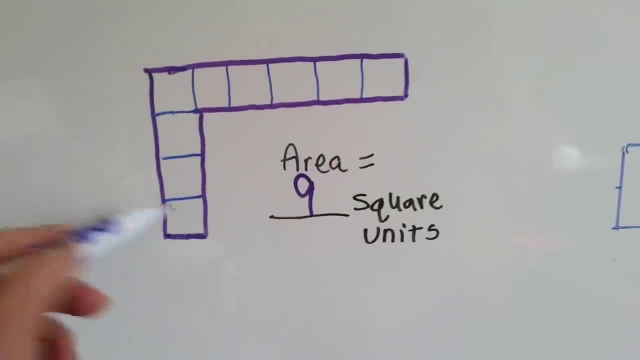 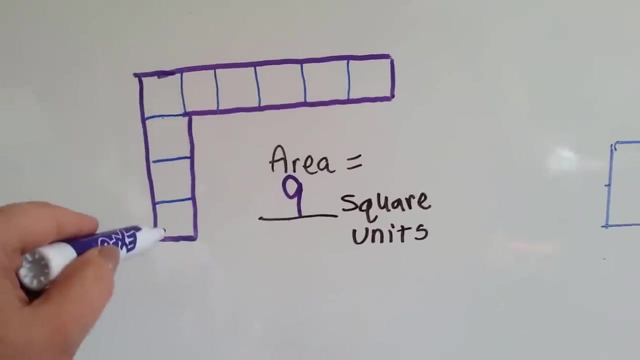 this funky L shape See. So its area is 9 square units. Now, if these were each 1 foot in size- and let's say it was outside and we were making a hopscotch or something and this was 1, these were each 1 foot in size. they would be 9 square feet. If it was inches. 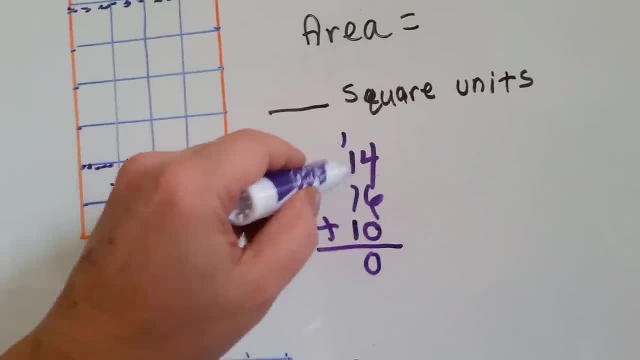 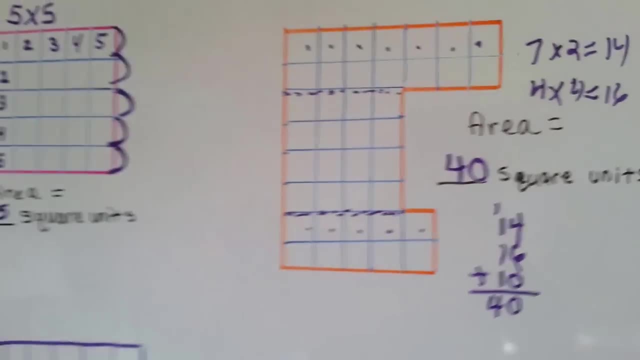 4 and 6 is 10.. We're going to carry the 1 and put the 0 down. 1, 2,, 3, 4.. There's 40 square units here. see Now. remember we weren't able to just do length times width like this one, because it was. 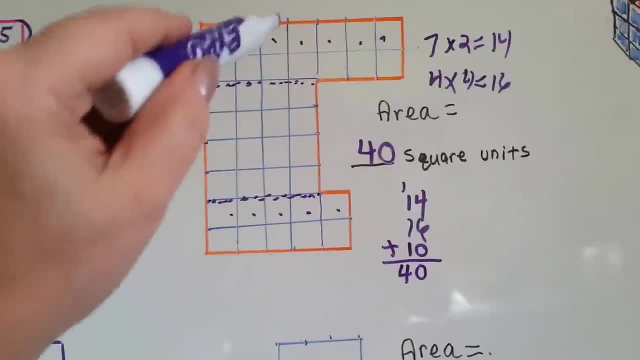 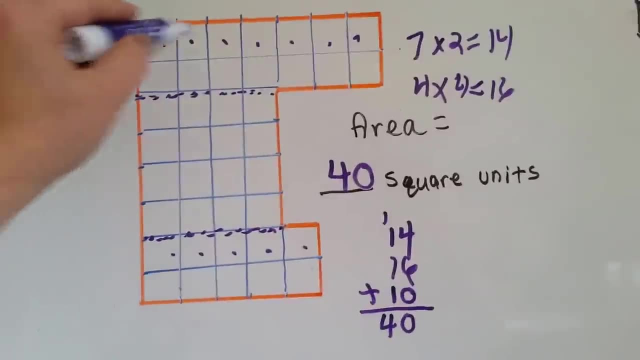 all full. This one's got a missing space here. So what we did was we broke it into sections and did it that way. Now we didn't even have to do times table. We could have just added up, you know, 7,, 8,, 9,, 10,, 11,, 12,, 13,, 14,, 15,, 16,, 17,, 18,, 19,, 20,. 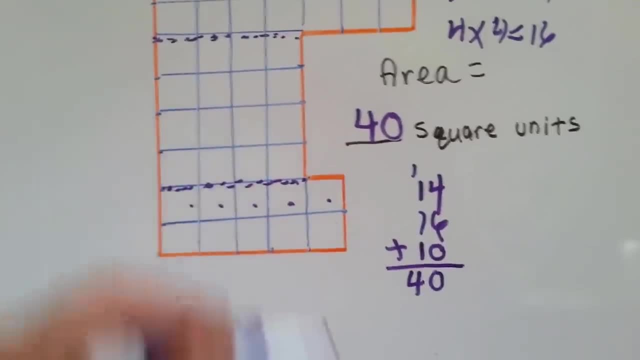 21,, 21,, 22,, 23,, 24,, 25,, 26,, 27,, 28,, 29,, 30,, 31,, 32,, 34,, 35,, 36,, 37,, 38,, 40,, 42,, 43,. 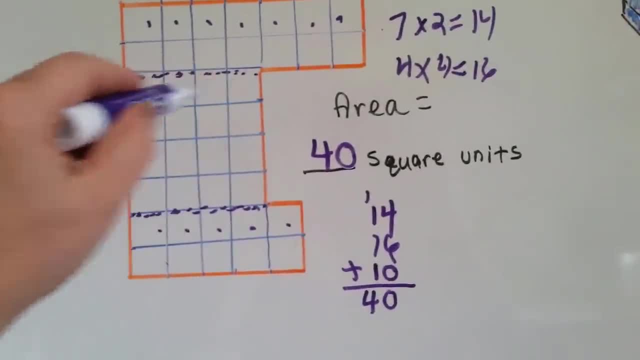 44,, 45,, 46,, 47,, 48,, 49,, 50.. We could have done it this way and counted each one of these separately. It's just a little quicker to go like this and like this with the length and the width. 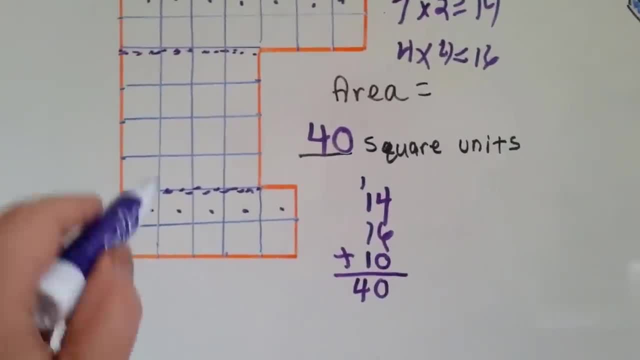 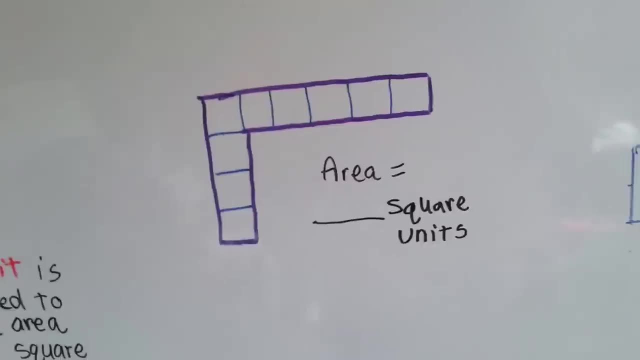 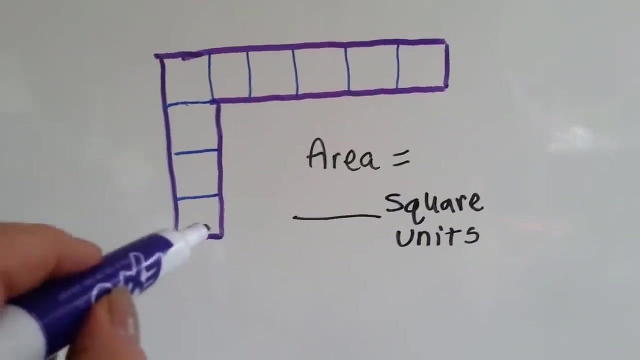 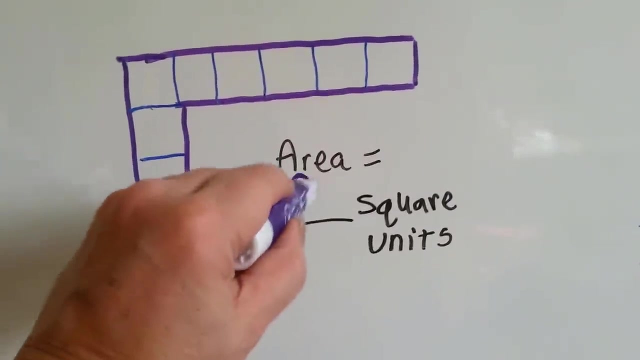 and multiply it and then get the amount. Just make sure that you break it off wherever it looks like it's changing. okay, Now let's look at this over here. What is the area of this? What are the unit squares? This one's got 1,, 2,, 3,, 4,, 5,, 6,, 7,, 8,, 9, 9 square units, and this one we were just 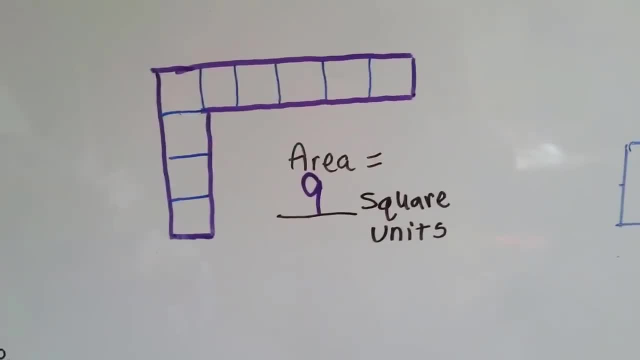 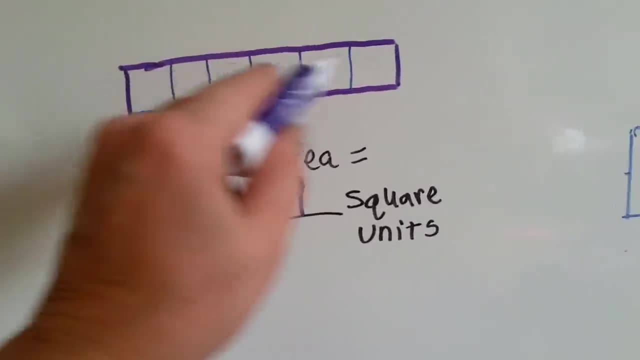 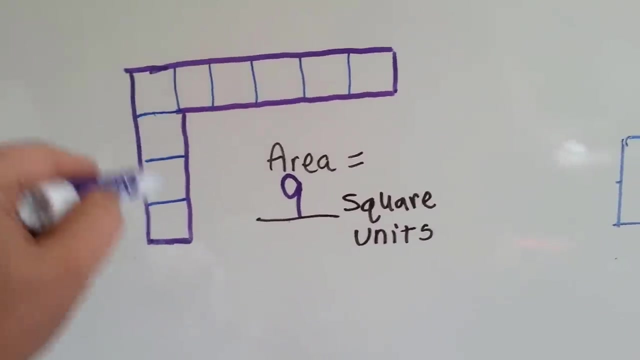 able to count because it's in this funky L shape, see. So its area is 9 square units. Now, if these were each one foot in size- and let's say it was outside and we were making a hopscotch or something and this was one- these were each one foot in size- they would 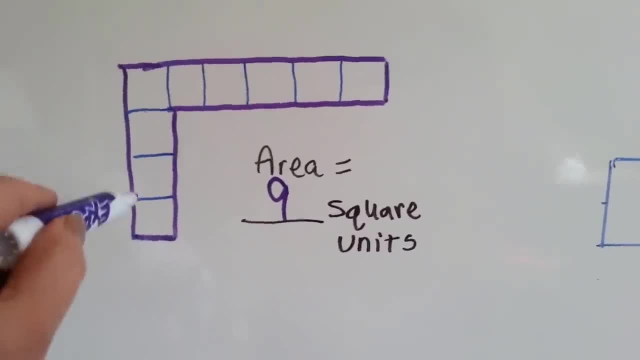 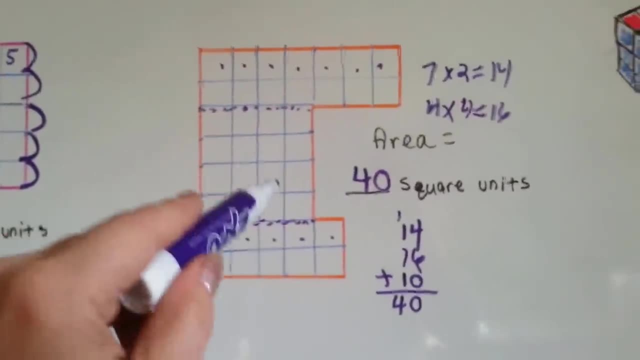 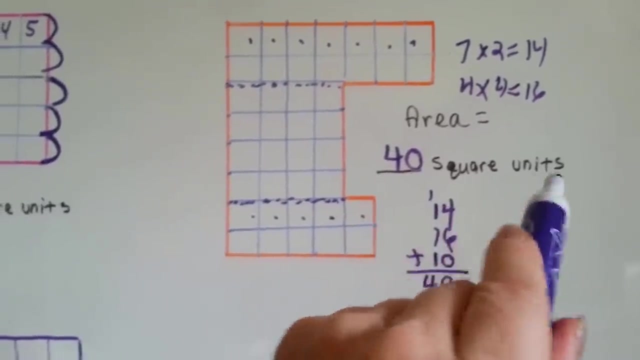 be 9 square feet. If it was inches, it would be 9 square inches, Same with these. If it was what? if this was a huge piece of land and the house was on it and these were each miles, We could say there were 40 square miles. see. 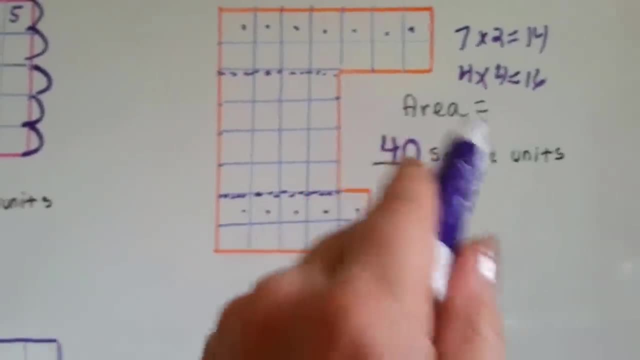 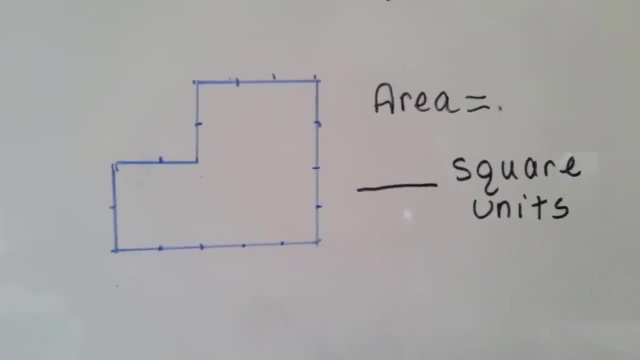 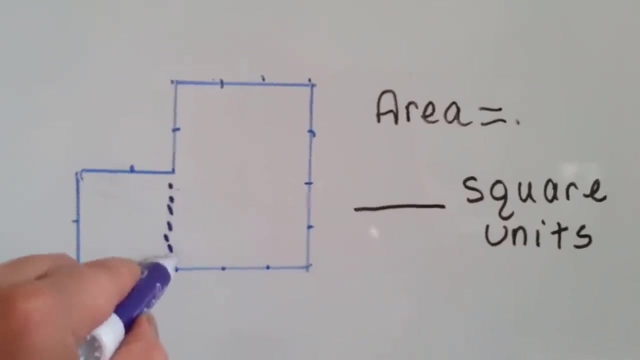 So, depending on what the measurement is that we're using, that's what the square unit is Now. can you look at this one without the lines and figure out how many square units are in this one? Can you figure it out How many do you think are in this section right here? 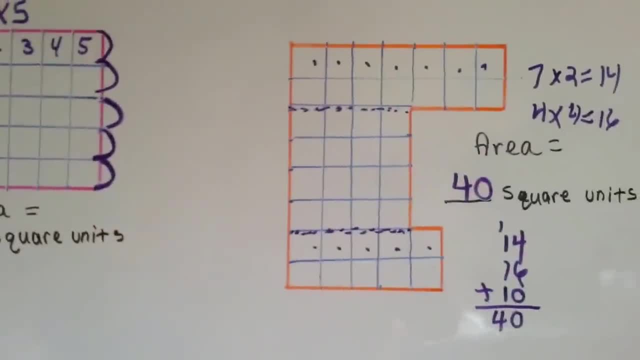 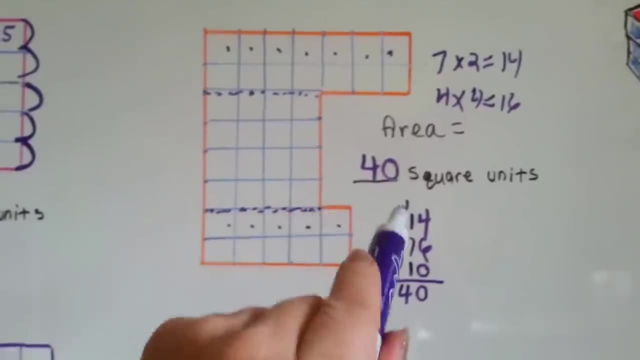 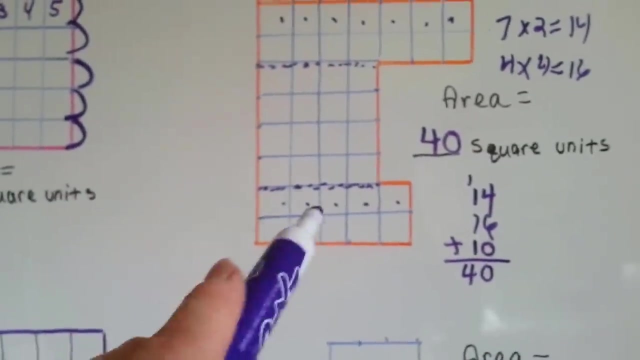 it would be 9 square inches. Same with these. If it was …. what if this was a huge piece of land and the house was on it and these were each miles? We could say they were 40 square miles, See. So, depending on what the measurement is that we're using, that's what. 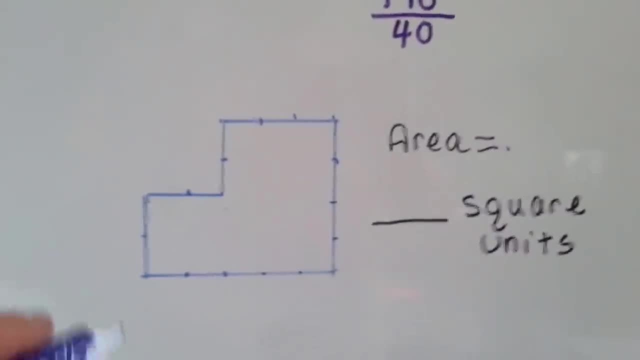 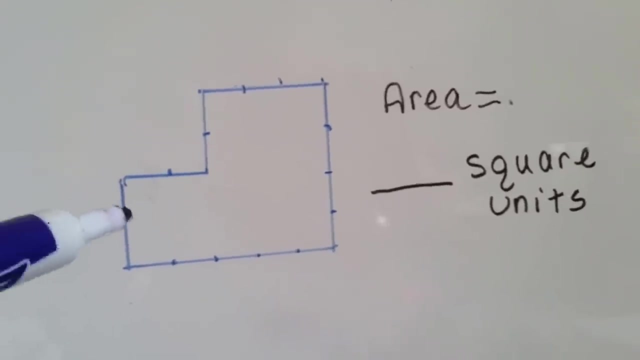 the square unit is Now. can you look at this one without the lines and figure out how many square units there are in this one? Can you figure it out How many square units are there in this one? How many square units are there in this one? How many? 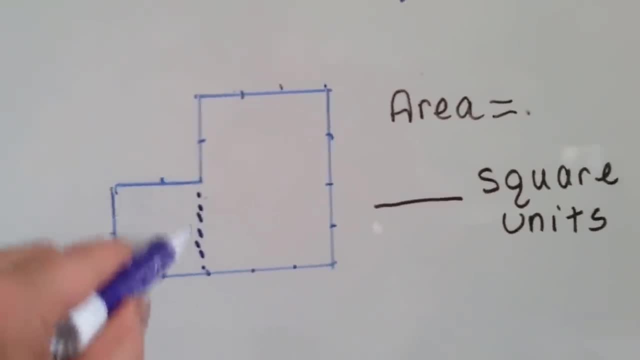 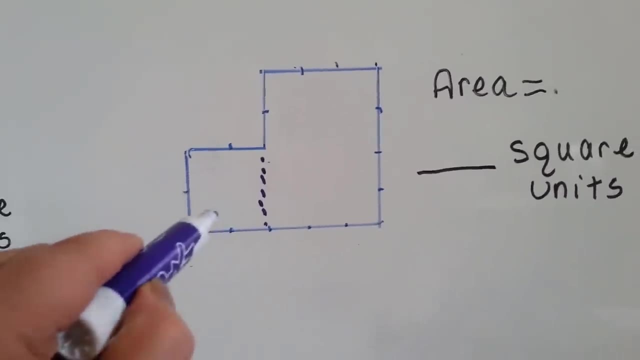 how many square units are there in this one? How many square units are there in this one, How many you think are in this section? right here Can you see how many you think might be in this section here: One, two, three, four. So there's four in this little area here. 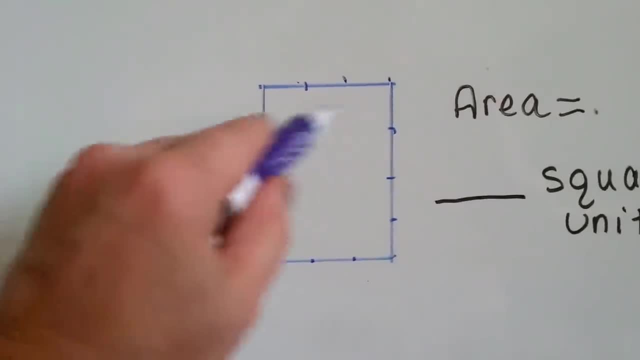 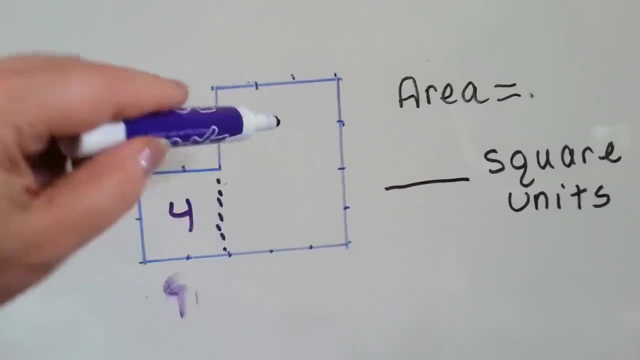 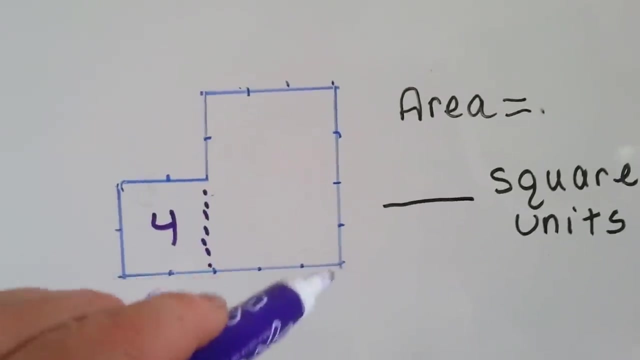 There's four inside of there And how many would be inside of here? There's one, two, three units. See the little dots. There's three units going across And how many are coming up and down? One, two, three, four, Three times four is Three times four is twelve. 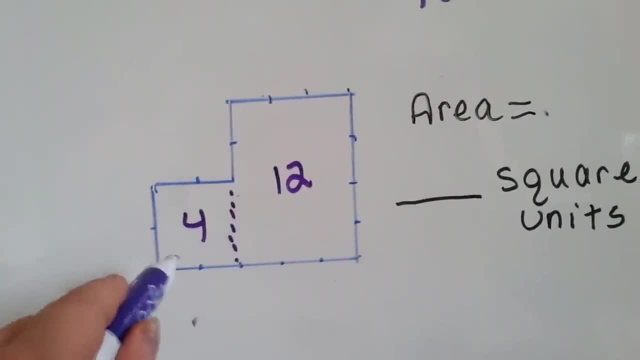 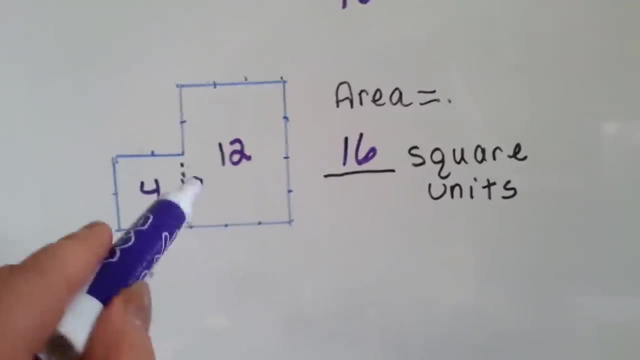 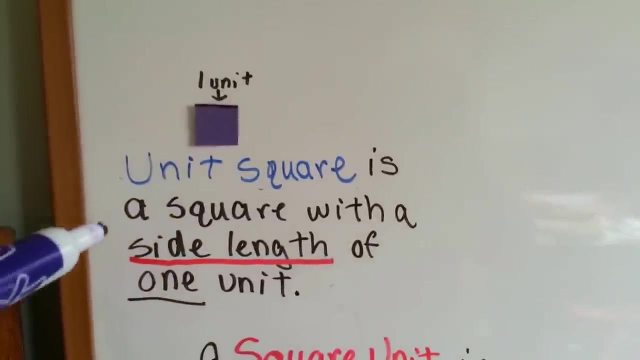 And now we can add the two sections together. Four plus twelve is Four plus twelve is sixteen, So there's sixteen square units in this shape, right here. Okay, So what you need to remember is a unit: square is just a square. 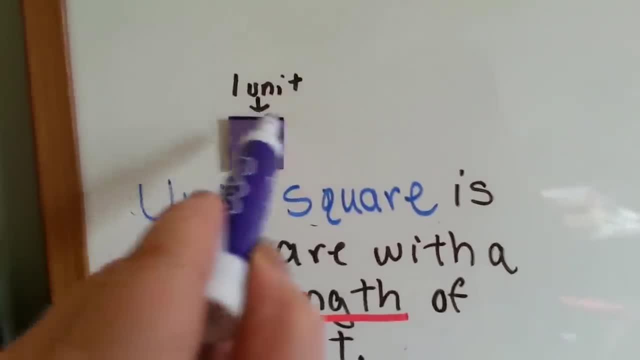 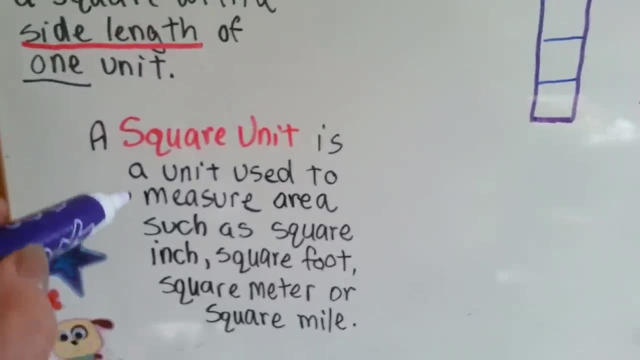 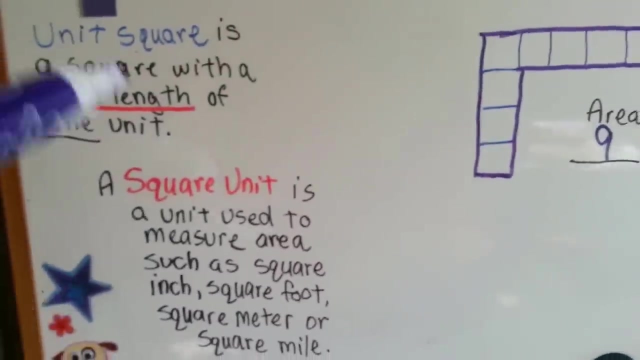 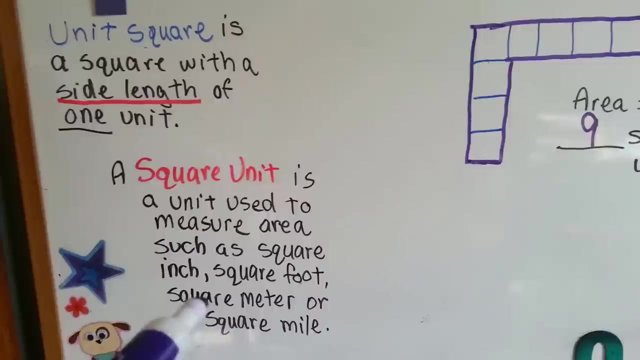 A square unit is anything like this, with a side length of one unit. Okay, A square unit is a unit used to measure areas such as square inch, square foot, square meter, square mile. so there is a difference between the two, Because the square unit 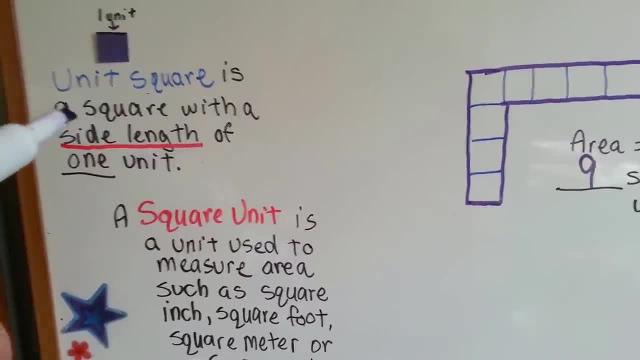 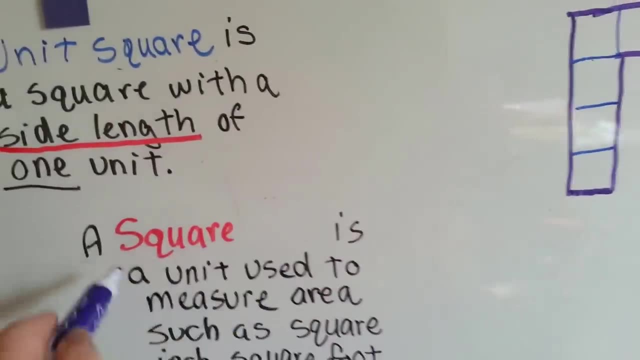 actually uses a measurement of about a centimeter or a meter where a square. it could be anything, It could be anything. It's just a unit, okay. The reason, in fact, is: Well, it's not a reason, but we shouldn't even put unit after this. 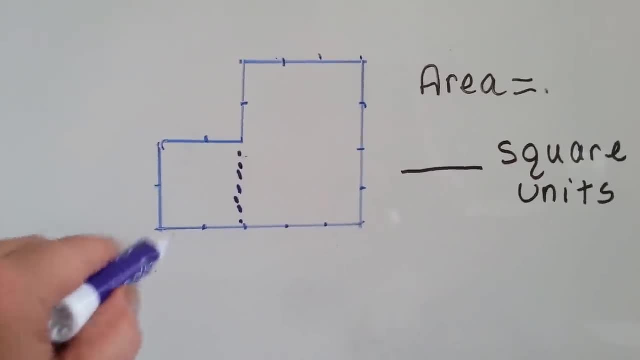 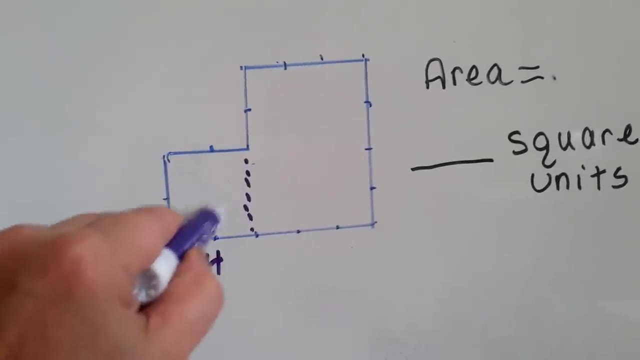 Can you see how many you think might be in this section here? 1,, 2,, 3,, 4, so there's four in this little area here. okay, there's four inside of there, and how many would be inside of here? 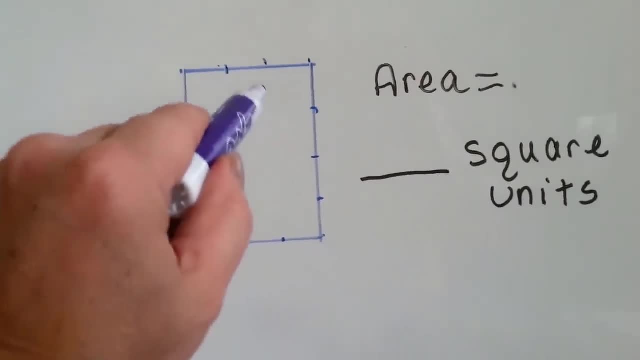 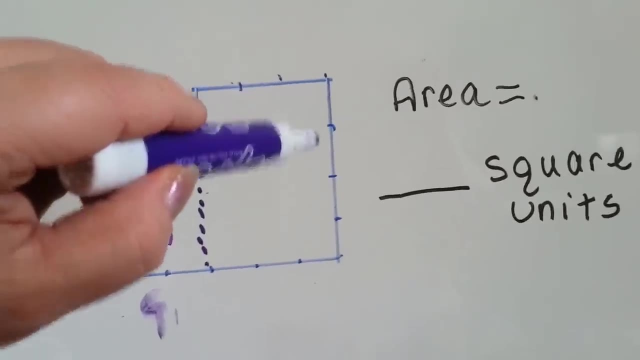 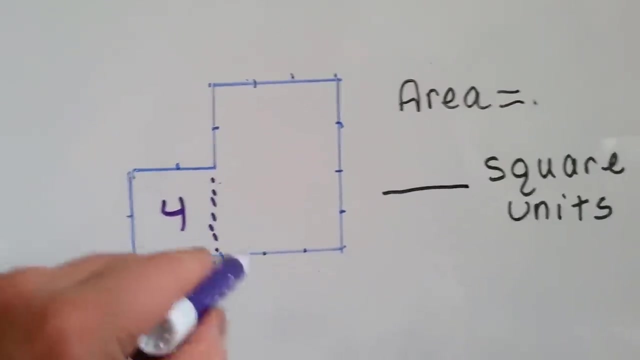 Okay, there's 1,, 2,, 3 units. see the little dots. There's three units going across and how many are coming up and down? One, two, three, four, Three times four is Three times four is twelve. 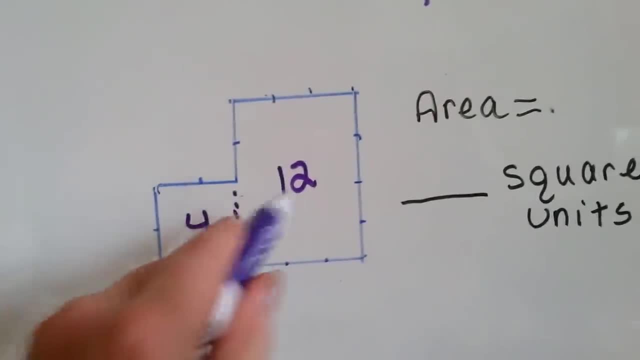 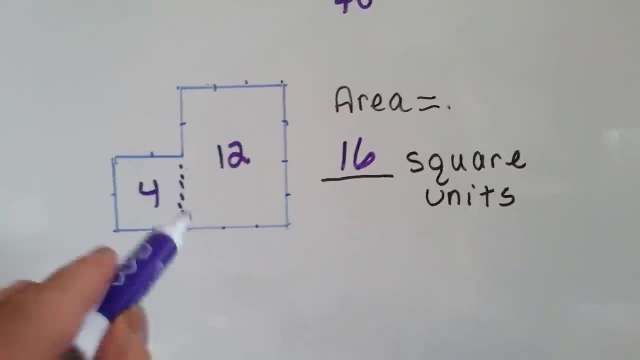 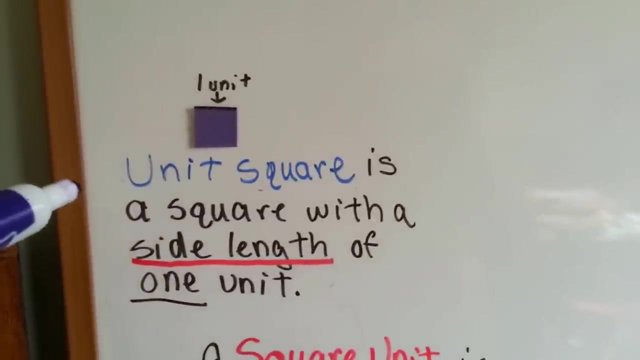 And now we can add the two sections together. Four plus twelve is Four plus twelve is sixteen, So there's sixteen square units in this shape, right here. okay, So what you need to remember is a unit. square is just a square, like this: 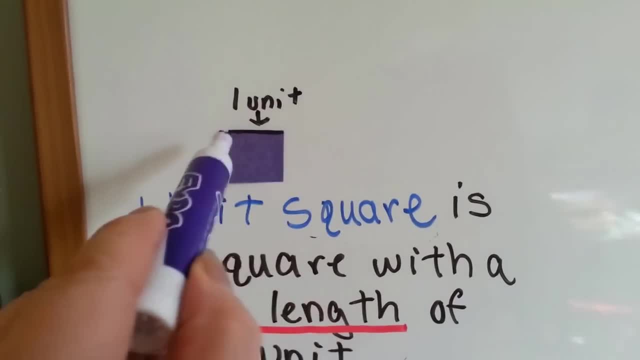 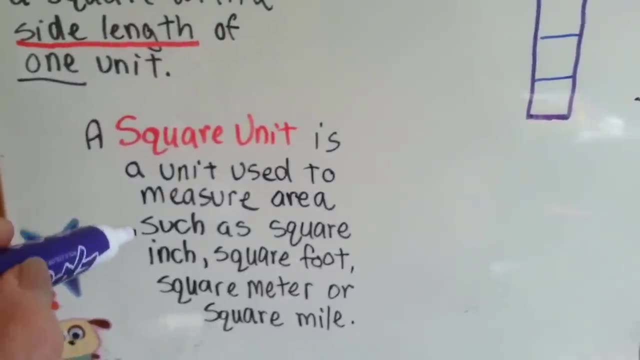 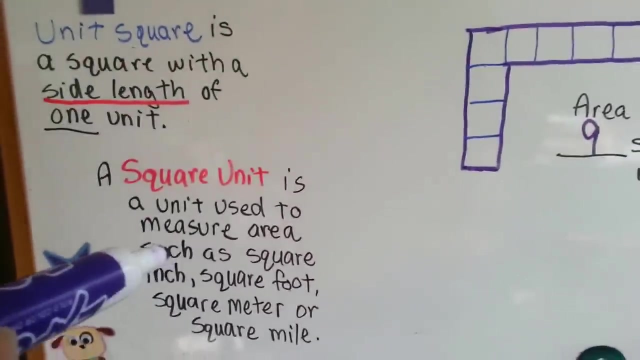 with a side length of one unit. okay, The side of it is one unit, alright. A square unit is a unit used to measure areas such as square inch, square foot, square meter or square mile. So there is a difference between the two. 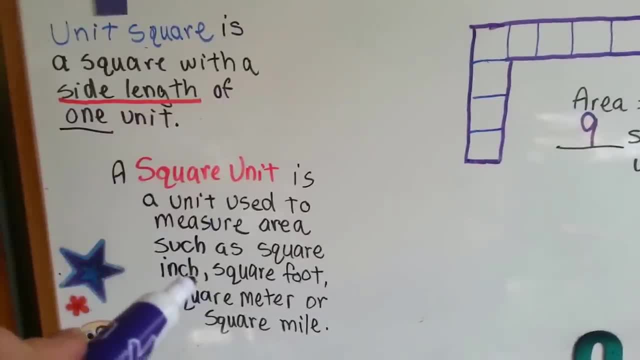 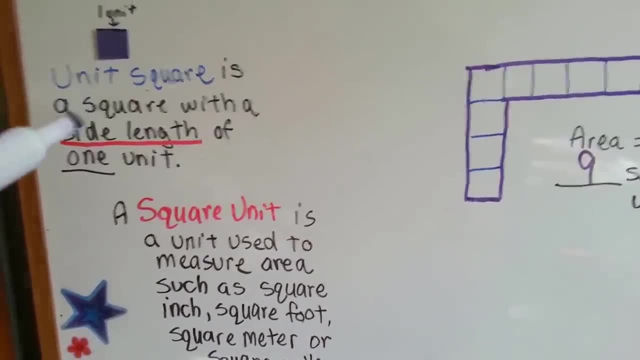 because the square unit actually uses a measurement like an inch or a centimeter or a meter, where a square unit could be anything. It could be a crayon, it could be a paperclip, it could be anything. It's just a unit, okay. 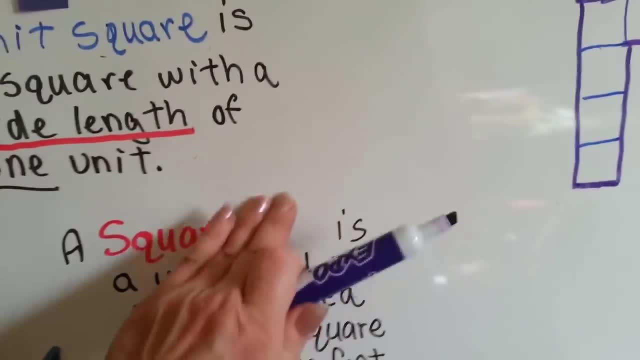 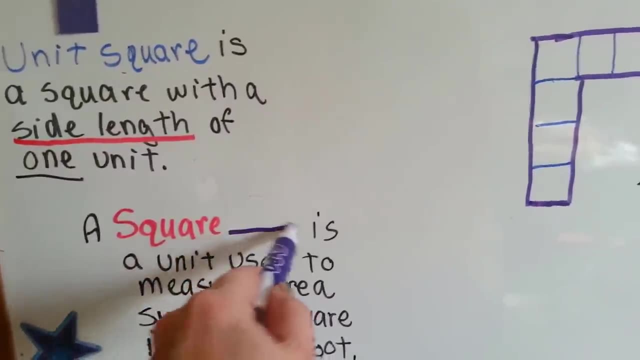 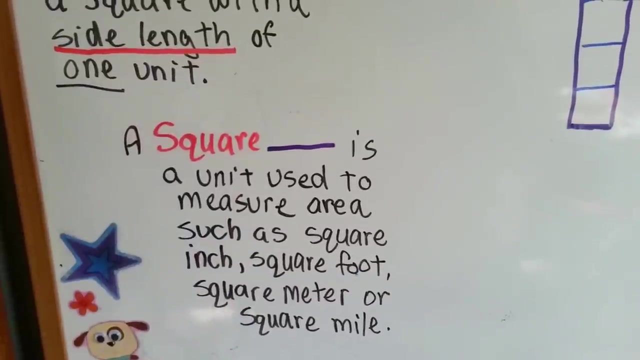 The reason, in fact, is: Well, it's not a reason, but we shouldn't even put unit after this. It should be square something. It should be square, centimeter, inch, mile, square block. okay, Square inch, square foot. 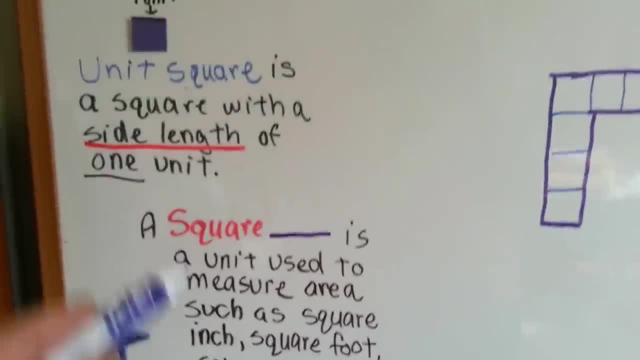 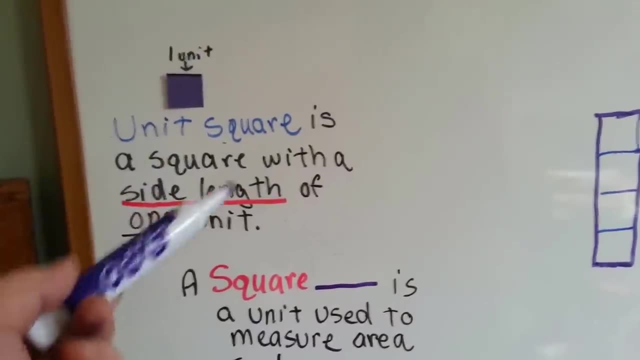 That's actually what this should say, instead of square unit. A unit square is any size square that you're using to measure as one unit. like I said, like a crayon or a paperclip, This is actually a square inch, a square centimeter, see.